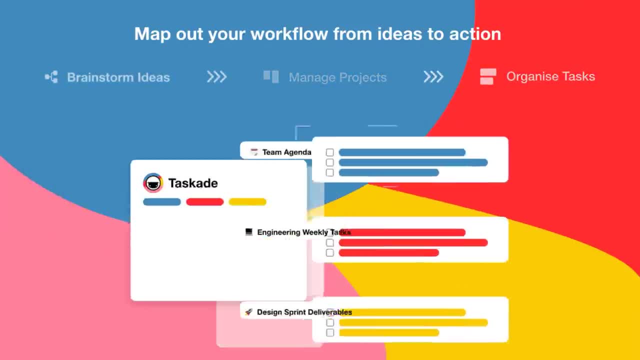 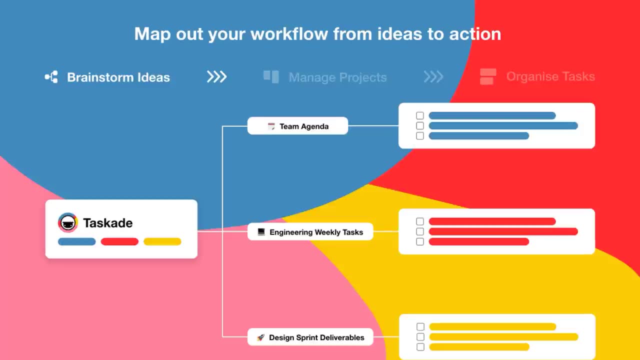 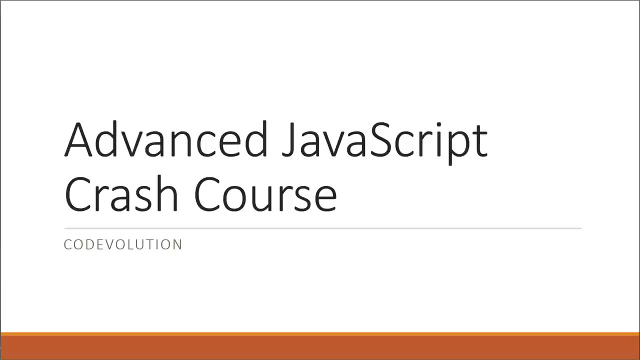 This video is sponsored by Taskade, a real-time organization and collaboration platform. Make sure to check the description for a discount on your subscription. Hey everyone, my name is Vishwas and welcome to this crash course on advanced JavaScript. In this crash course, we will understand some of the advanced topics in JavaScript. 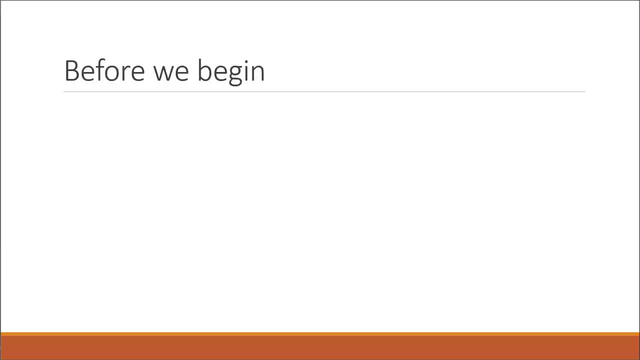 Before we begin, let me go over a few points. First, I would like to mention this course is a continuation of the JavaScript Fundamentals crash course. If you are new to JavaScript, please watch that video before proceeding. Also, if you are someone who is already familiar with advanced JavaScript concepts, 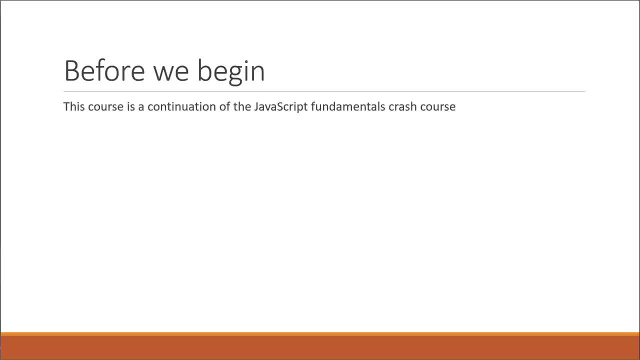 I would suggest you wait for the asynchronous JavaScript crash course. Second, we are going to cover concepts that you, as a front-end developer, should know. It is not an exhaustive list, but the topics we will cover are required for any front-end interview you might appear for, and most of the topics 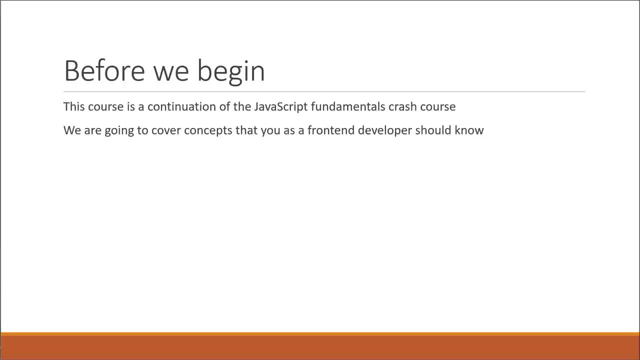 also find daily usage in your work as a developer. So we will be covering a limited number of topics, but they all are very important. Third, this video, unlike other videos in my channel, is a crash course and is longer in length. 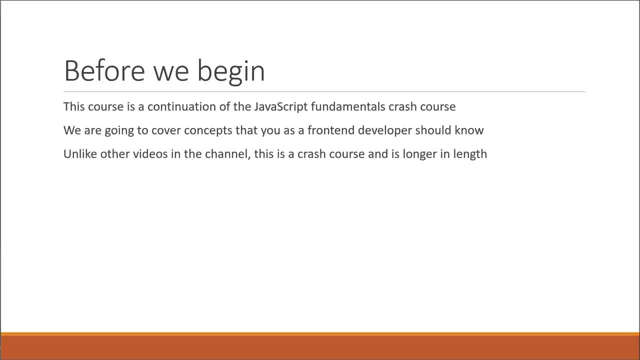 That doesn't mean you have to sit through the entire video at once. Take it easy, pause when necessary and, most importantly, make sure you code along with me, as that is the best way to learn. By the end of this video, you will have a solid understanding of the advanced concepts in JavaScript. 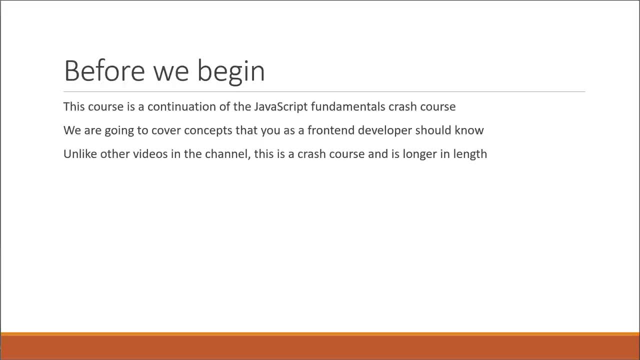 All right, with these points in mind, let's go over the topics we will be learning in this video. We're going to start off from the first topic where we left off in the fundamentals crash course, and that is about scope. We will specifically look. 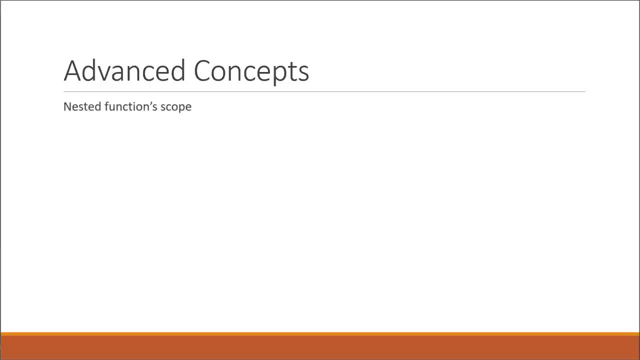 at nested functions scope, which will then take us to understanding closures in JavaScript. Next, we will learn about the concept of currying. This is followed by the all-important this keyword. We will then learn about prototype and prototypal inheritance. That is followed by learning about 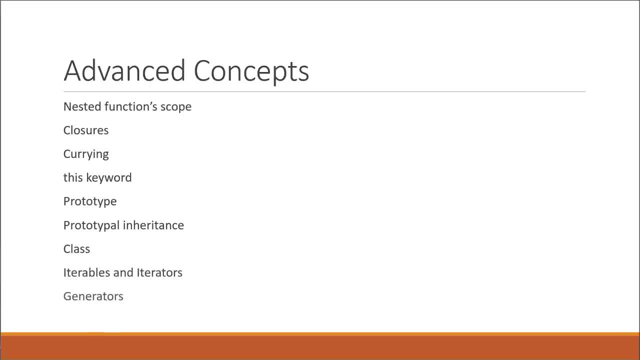 classes, iterators and, finally, generators. We will save the async JavaScript concepts for the next video. If you have had difficulty understanding any of the listed topics here, then you are at the right place. Now, then, for some setup. We are going to reuse the setup from the previous crash. 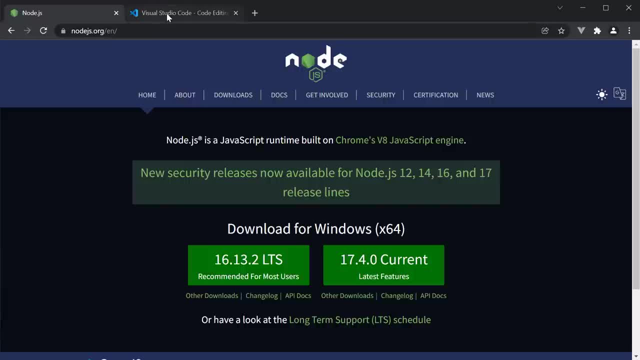 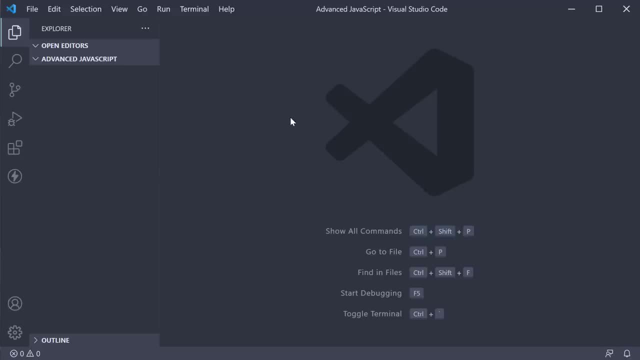 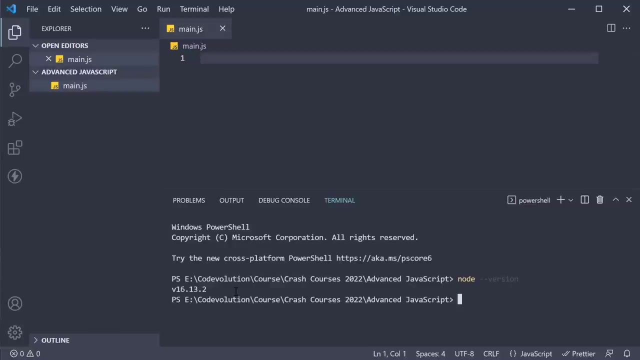 Open VSCode inside a folder of your choice. I have created a folder called Advanced JavaScript and within the folder create a file called Mainjs. Open the terminal, So view terminal and run node-oddsjs. and run the file dash version. if you see the version number in your terminal, we are good to go, all right. 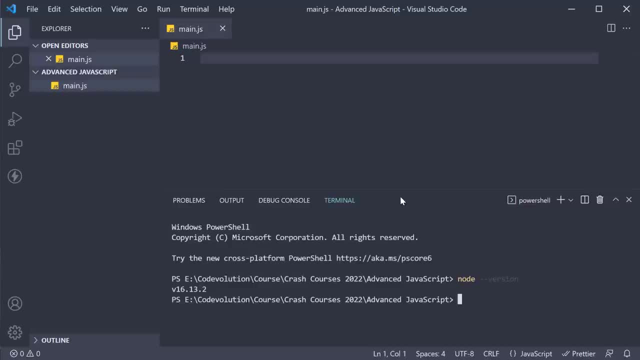 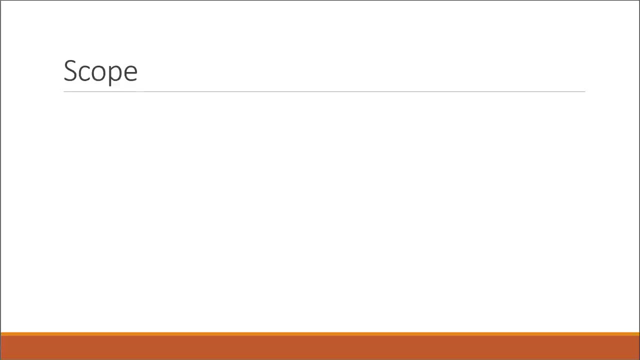 let's begin by revisiting the concept of scope in javascript. in the fundamentals crash course, we learned about three types of scope: block scope, which dictates that variables declared inside a pair of curly braces cannot be accessed from outside. the block function scope, which dictates variables declared inside a function cannot be accessed from outside. 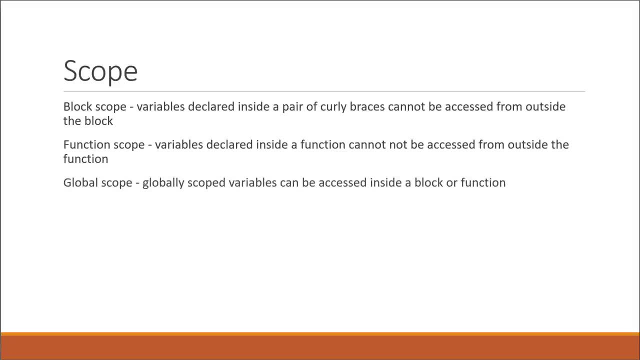 the function. and finally, global scope, which is the scope outside a top level block or function of code. we also learned that globally scoped variables can be accessed inside a block or function. we also had a look at examples related to each of these scopes, in case you missed it, please. 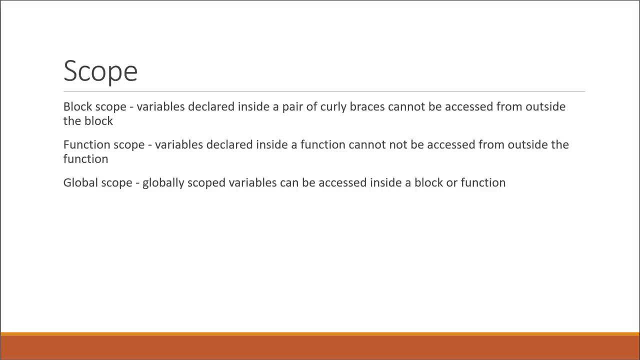 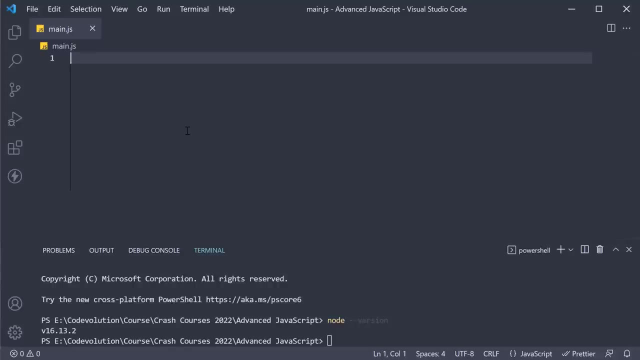 watch the last episode of chop paintings: 10 to 15 minutes of the fundamentals crash course for continuity. Now in the advanced crash course, let's learn about a nested functions scope with an example In mainjs. let's declare a variable a and initialize it to 10 in. 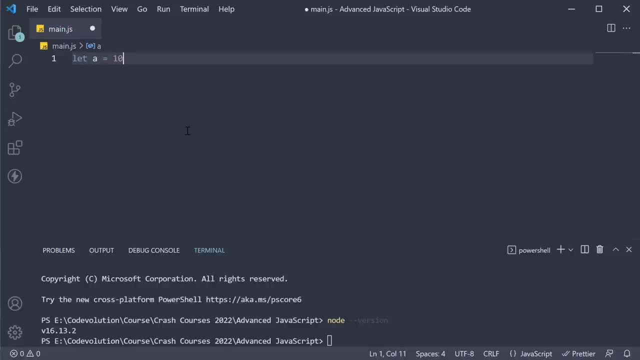 the global scope. Next, let's define a function called outer and, within the body of the function, define a variable b and initialize it to 20.. Within this function, let's define another function called inner. and yes, in JavaScript it is possible to define a function within a function, So function. 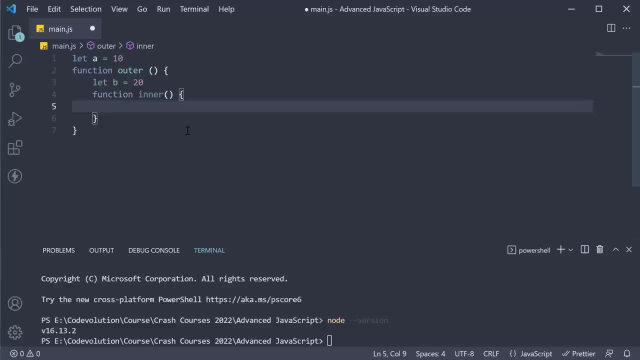 inner and within the inner function, let's declare another variable, c, and initialize it to 30. We then log a, b and c to the console within the inner function: a, comma b, comma c. Next, within the outer function, we invoke the inner function. Finally, we invoke the outer function If we save the file and run the. 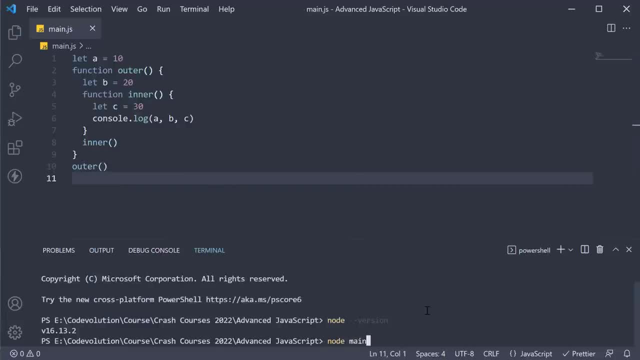 code main. what do you think is logged in the terminal? You can see the output is 10, 20 and 30.. Let's understand this output from the JavaScript engine point of view. We can directly dive into the log statement on line 6.. JavaScript basically has to: 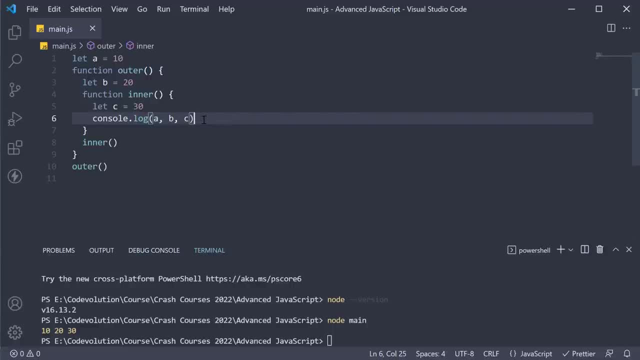 look up for values of a, b and c. Let's start with c. JavaScript checks if c is defined in the inner function scope. It is, and its value is 30.. So 30 is logged in the terminal. Next it looks for b. It checks if the variable b is available in the inner function scope. 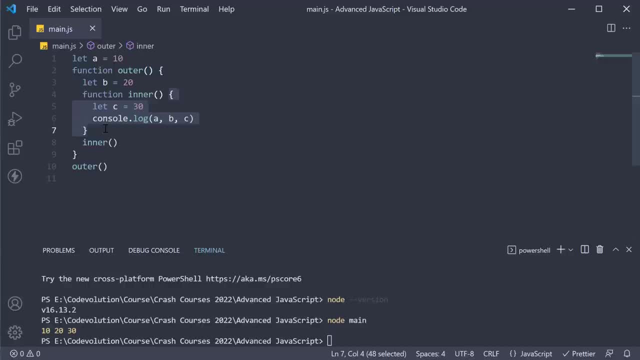 It is not. So it goes one level up and checks in the outer function scope Is the variable b present in the outer function scope and its value is 20.. So 20 is logged in the terminal. Finally, we have the variable a. 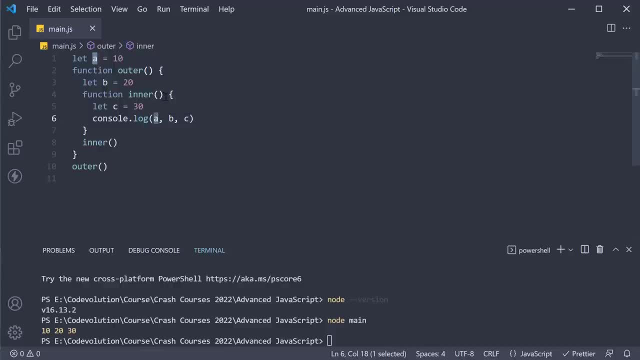 JavaScript checks if the variable is present in the inner function scope. It is not, It then checks if the variable is present in the outer function scope. It still doesn't find it, It moves one more level up and reaches the global scope. It checks again if the variable is present in the 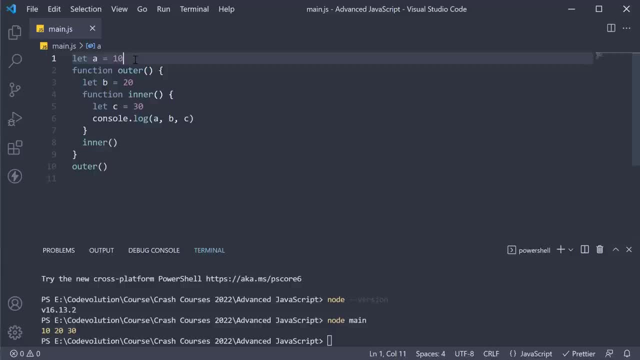 global scope. It is, and its value is 10,, which is logged to the terminal. So the resulting output is 10,, 20, and 30.. Now this is an example of lexical scoping, which describes how JavaScript resolves variable names when functions are nested. 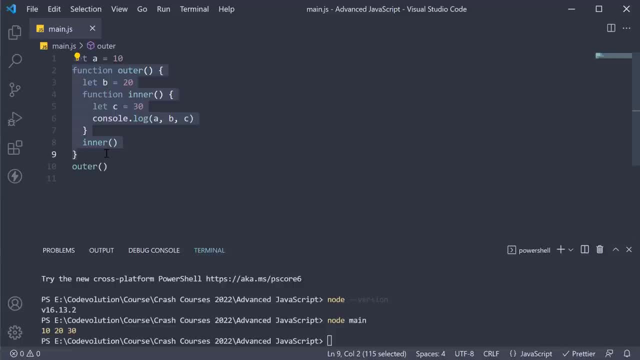 When we have nested functions, JavaScript variable lookup starts with the innermost function, where we are trying to access the variable, and moves outward until it reaches the global scope. But the bottom line I want you to remember is that nested functions have access to variables declared in their own scope as well as variables declared in the outer scope. 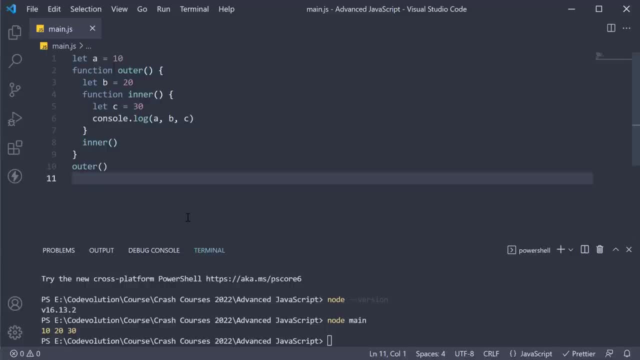 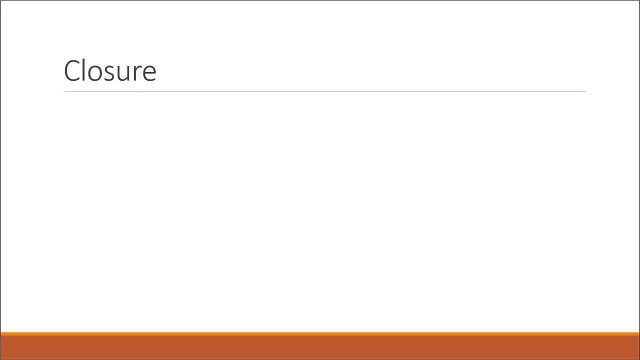 All right, with this understanding of nested functions scope, we are now ready to proceed to the second concept in this advanced JavaScript crash course, which is closures. Now, what exactly is a closure? According to Mozilla docs, a closure is the combination of a: 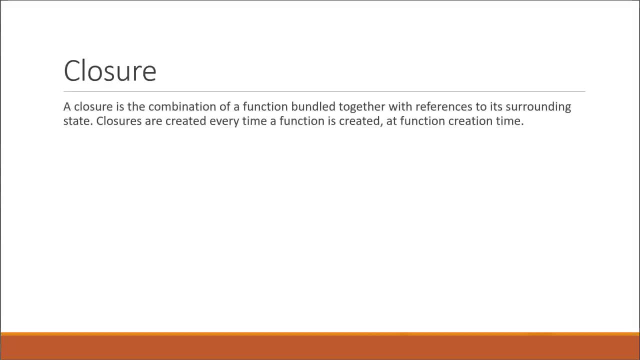 function bundled together with references to its surrounding state. Closures are created every time a function is created at function. Now let's look at some other examples of closed cases. In the example that we just saw, there is a closure in JavaScript. 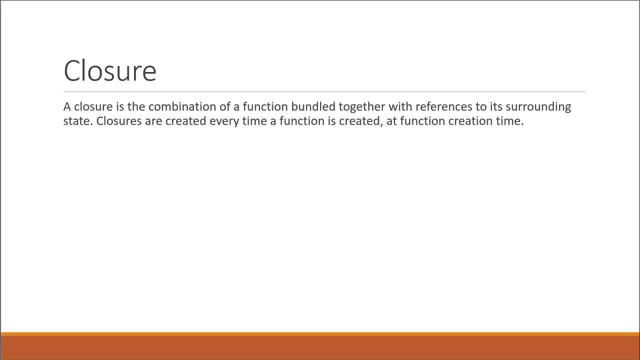 In the example that we just saw, there is a closure in JavaScript. Now, most of the time, a closure is when a function on the content of a function is collapsed, and when a function of a function is leaking, the function is closed. 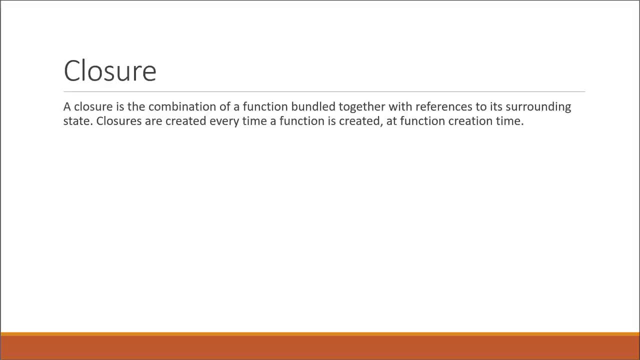 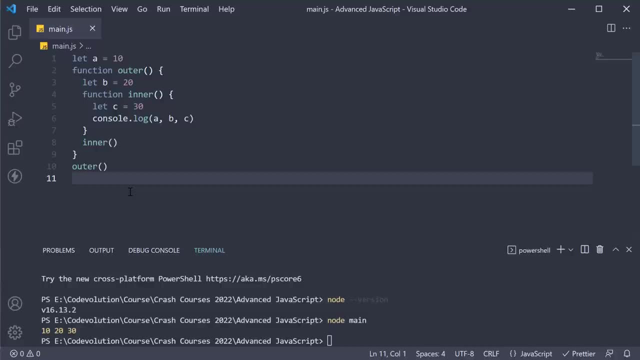 And this is because, as we saw in the example, there are only a few functions in the function. For example, example about nested function scope- we learned that nested functions have access to variables declared in their own scope as well as variables declared in the outer scope. let's now look at a 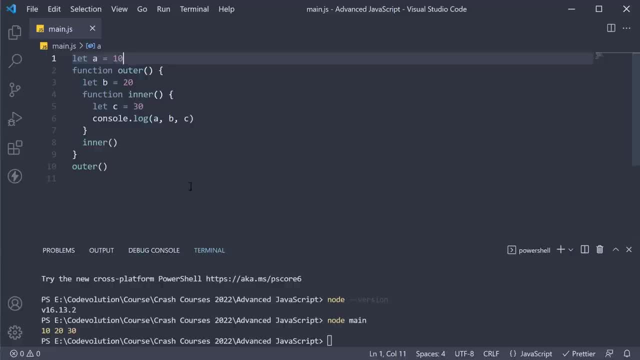 more simplified version of this example. comment out the code we have written so far. let's start over. we define a function called outer. within the function body, we declare a variable counter and initialize it to zero. we also define a nested function called inner, where we increment the value of counter. 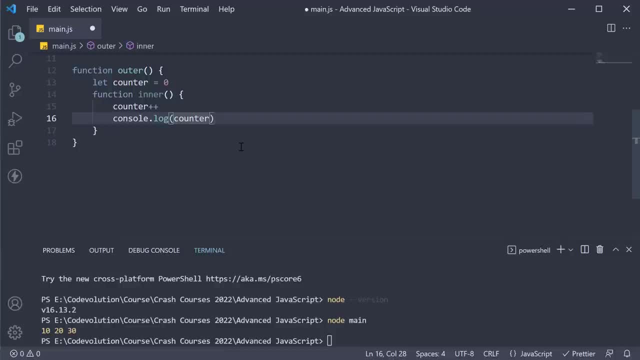 and then log that value right after the function definition. we invoke the inner function inside the outer function. finally, we invoke the outer function. now, if we were to run this code, what do you think is logged in the terminal node main? and we can see one. this should be clear by now because of how nested functions scope. 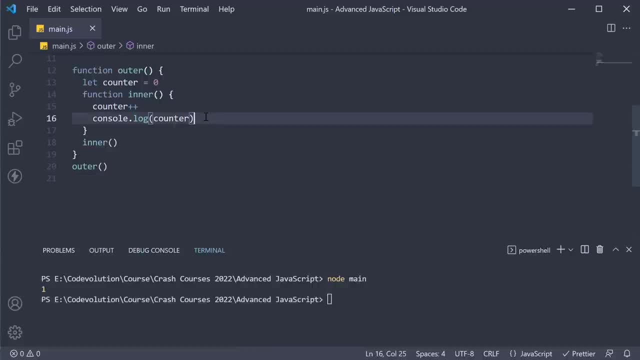 works in javascript. when the variable counter is encountered within the inner function, the javascript engine checks if counter is present in the inner function scope. it is not, it then checks the outer function scope. the variable is present and it increments the counter value by 1 and then the new value is. 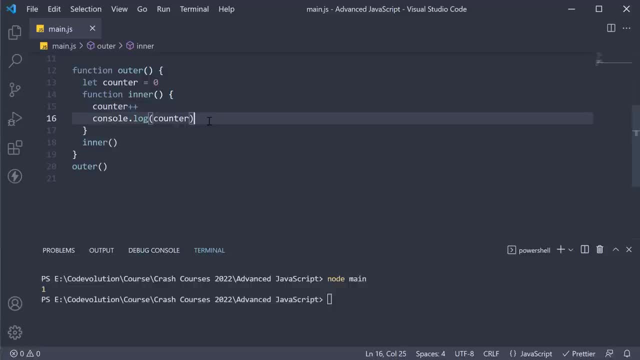 logged to the terminal, which is 1.. seems all right so far. now let's invoke the outer function twice. if you run the code, what do you think is logged in the terminal? the answer is 1 and 1.. this is because, with every new invocation of the function, 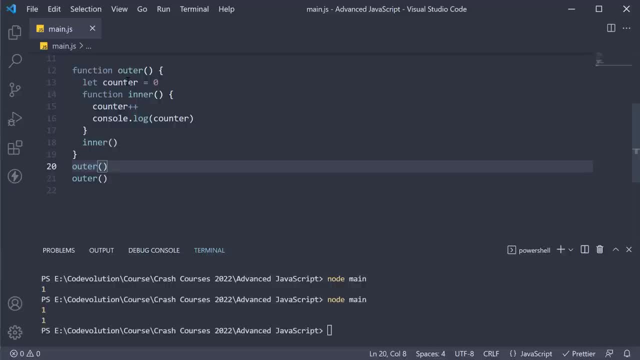 a temporary memory is established and we have a new counter variable initialized to 0 and then incremented. hence, every outer function call will always print 1 to the console. if this is clear, let's move on to a slight variation of this code. at the moment, we define the inner function and invoke it within the outer function. 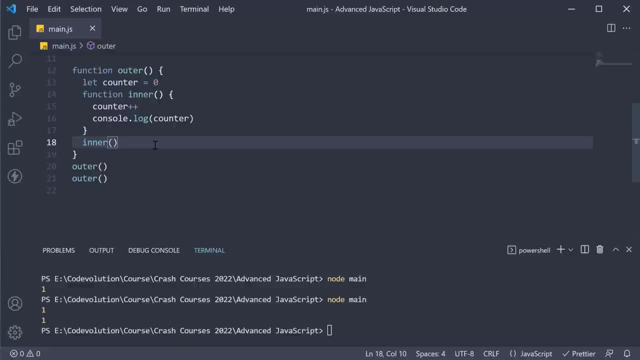 let's say we don't necessarily want to invoke the inner function right away. instead, we want to return the function and invoke it at a later point in time. in javascript it is possible to return a function from other functions, so let's return inner. in doing so we can assign the result of invoking outer function. 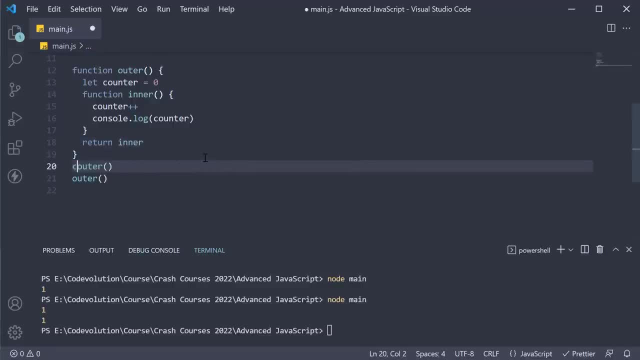 to a variable called fn. so const fn is equal to invoking the outer function, and this result is the inner function. so let us now invoke the fn function twice: fn parentheses. fn parentheses. remember: all we are doing is, instead of executing the inner function from within the outer function, we are returning it and then invoking the function twice. 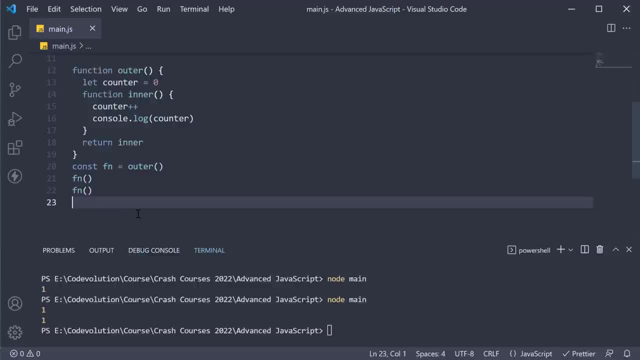 now, if we were to run the code, what do you think is logged to the console, node main, and you can see? the answer is 1 and 2.. now that's interesting, isn't it? we would expect the output to be 1 and 1, but it is 1 and 2.. 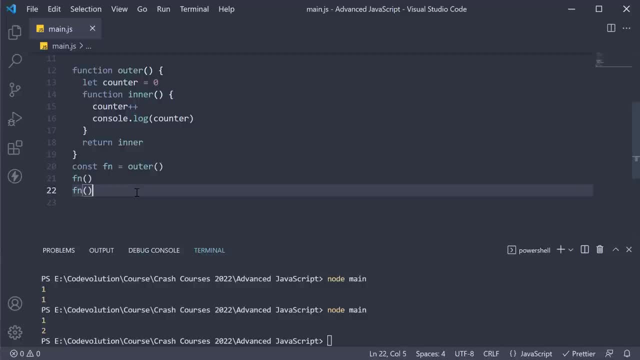 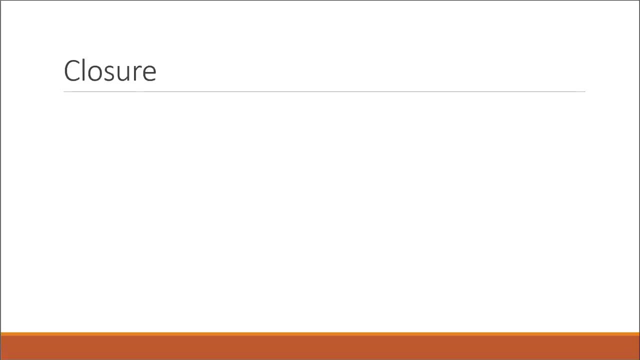 this is because of the concept of closures in javascript. here is a definition that i find is more easier to understand in javascript. when we return a function from another function, we are effectively returning a combination of the function definition along with the function's scope. this would let the function definition have an associated persistent memory which could hold 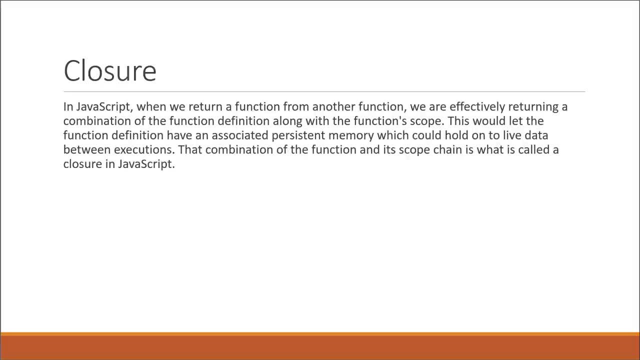 on to live data between executions. that combination of the function and its scope chain is what is called a closure in javascript. with this definition in mind, let's try to break down the example we have at hand now. i mentioned that a closure is created when a function is run. 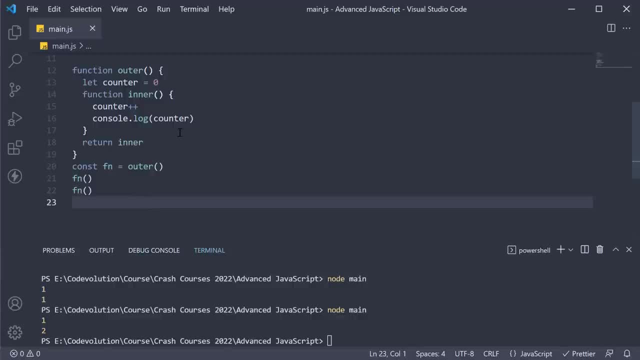 in a function, the function is returned from another function. if you take a look, that is precisely the scenario we have on line 18. we are returning the inner function from the outer function and, as it turns out, in such a scenario, javascript doesn't just return the inner function. 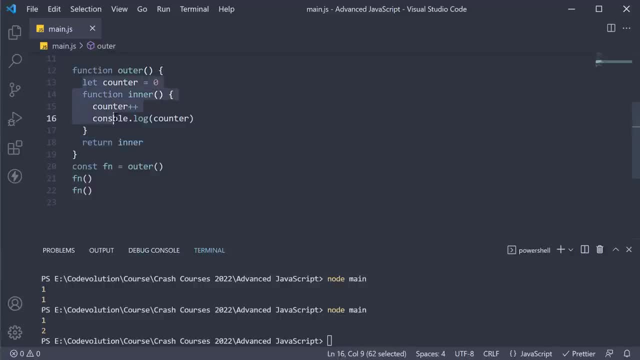 it returns the inner function as well as its scope. In our example, the function scope has just one variable called counter, initialized to 0. So we have the function inner bundled together with the variable counter, which is together termed as a closure, And in such situations the function will persist or remember the value of the counter variable. 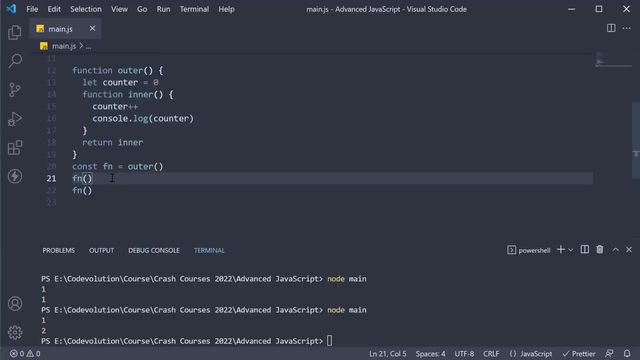 So, when we invoke the fn function for the first time, counter is incremented to 1 and the value is logged in the terminal. But the fn function, though, remembers that the counter value is 1.. So the next time we invoke it, it increments the counter value to 1 plus 1, which is 2.. 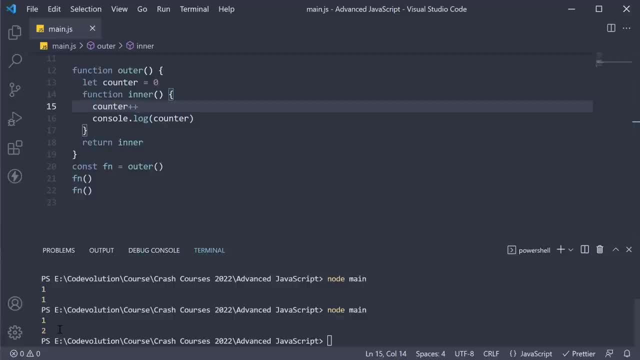 That is the reason we see output 1 and 2.. That is how closures work. The key point to keep in mind is that with closures, an inner function has access to variables in the outer function scope even after the outer function has finished execution. 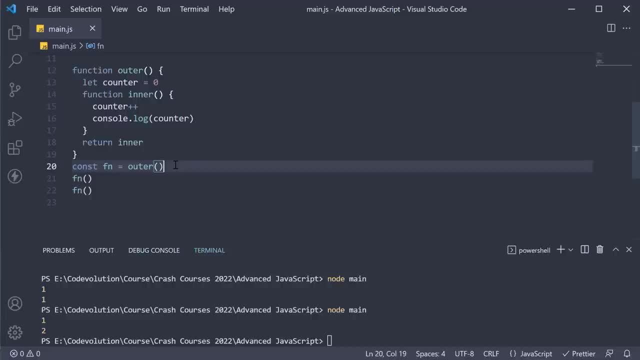 You can see in our example that when we invoke the outer function on line 20, it completes its execution, But the inner function still has access to counter variable, which is actually the outer function. So the inner function has access to counter variable, which is actually the outer function scope. 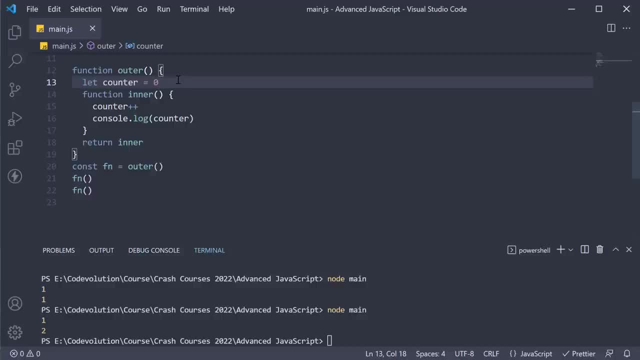 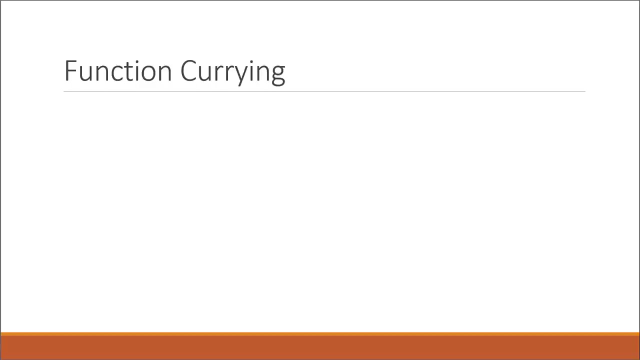 Now I get it. if this is a little difficult to understand, My advice would be to re-watch the concept 2 or 3 times and it will for sure start to make sense. Now, if you have understood closures, the next topic to learn is function currying. 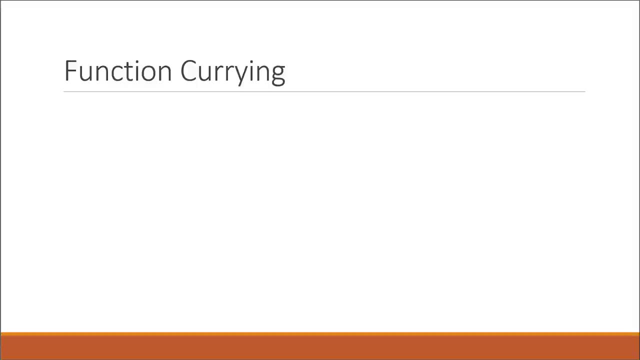 The best way to understand function currying is with an example. So that's the approach to function currying. So that's the approach to function currying. Let us start with the definition. What is function currying? Currying is a process in functional programming in which we transform a function with multiple arguments into a sequence of nesting functions that take one argument at a time. 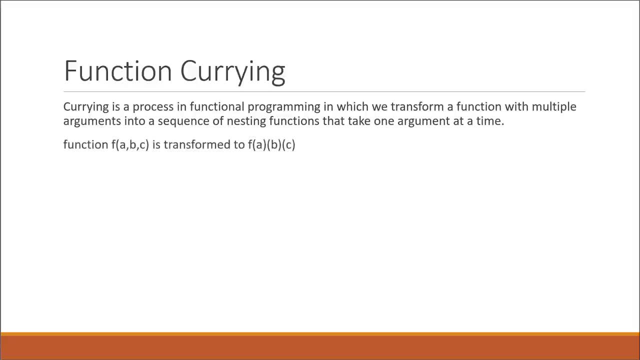 So if we had a function f of a comma b, comma c, we transform it into f of a of b of c. It is important to note that curry doesn't call a function, it simply transforms it. Let's head back to VS Code and understand this with a simple example. 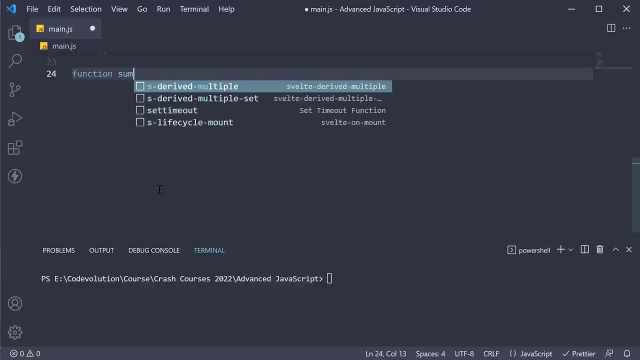 Let's define a function sum which takes three parameters- a, b, c- and returns their sum. To call or invoke this function, we write the function name, followed by parentheses, and within parentheses we specify the arguments. Let's go with 2,, 3,, 5, which correspond to a, b, c. 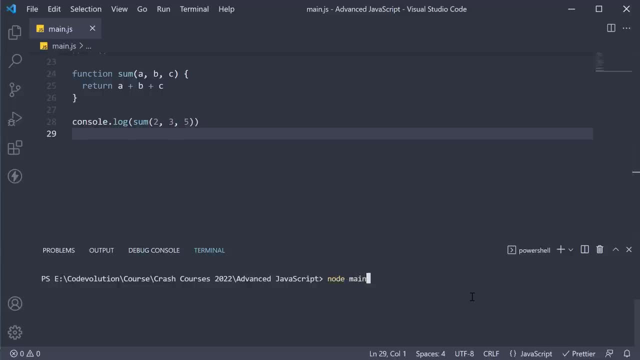 If we were to run this code, node main, we get the output 10.. Now currying this sum function means that we need to transform sum from calling it with all three arguments to calling it with one argument at a time. So from sum 2,, 3,, 5 we should transform it. 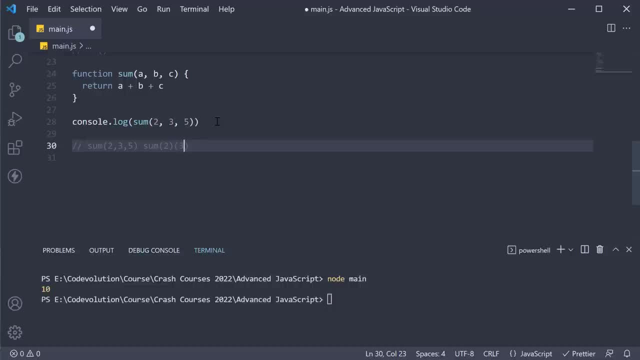 to sum 2,, 3,, 5, one argument at a time. The way we do that is by nesting functions, where each function takes three parameters- a, b, c- and returns their sum. Let's understand the code. We start off with a function called curry, and this function will accept a function as its argument. 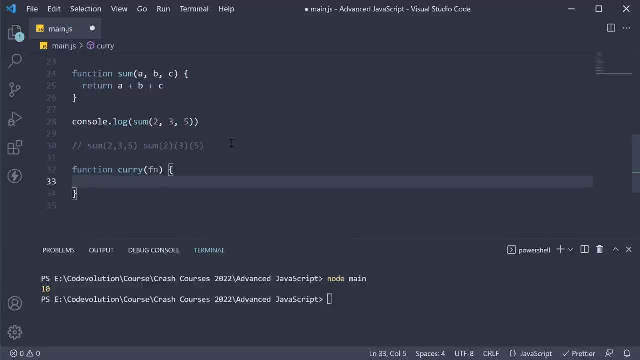 and return the curried version of the function For each of the three arguments. we return individual functions that accept one argument at a time and the functions will be nested one inside the other. So the curry function will return a function which accepts an argument a. 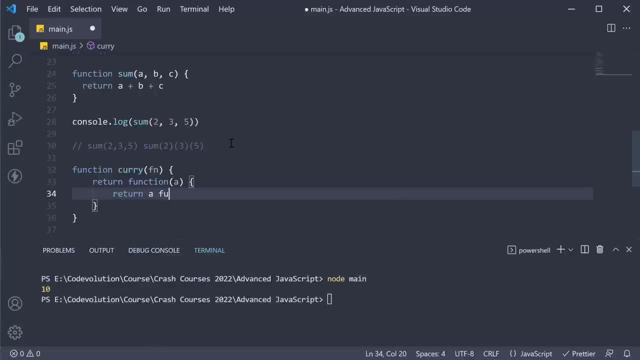 This function in turn will return a function which accepts argument b. This function in turn will return a function which accepts argument c. We are transforming from accepting three arguments at a time to one argument at a time Now when we have broken down the function into nested functions. 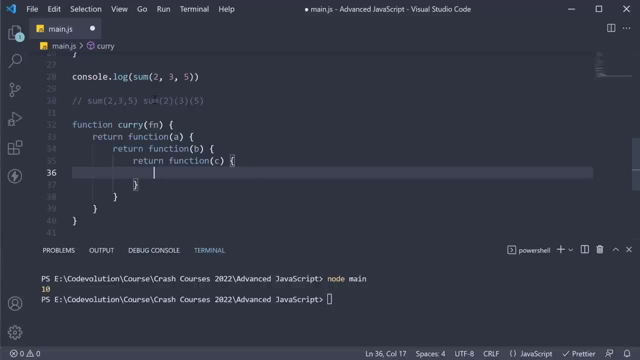 we check if we have all the necessary arguments to run the given function. In our case we have a, b and c, so we have all the arguments. So now, from the innermost function, we return the actual passed-in function with all the necessary arguments. 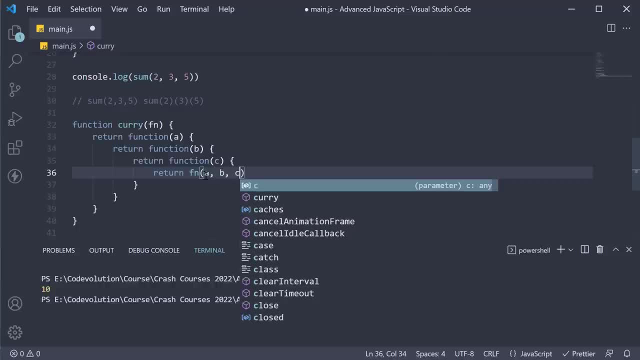 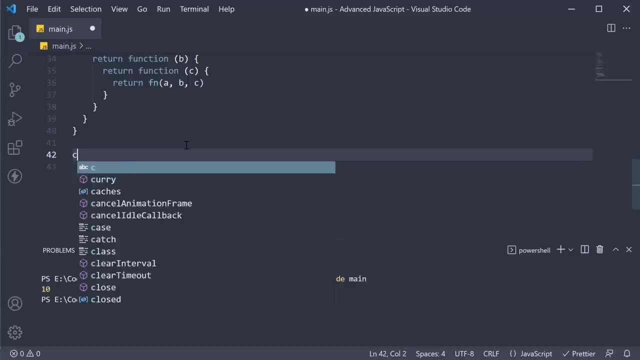 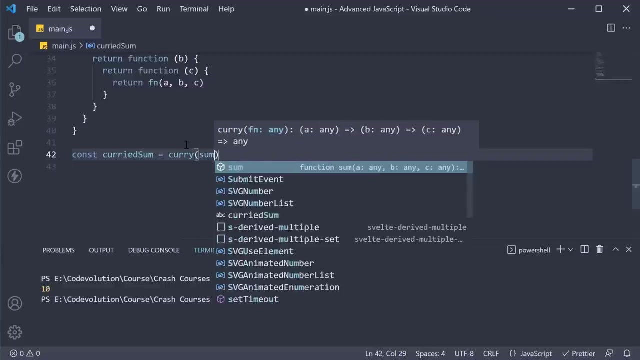 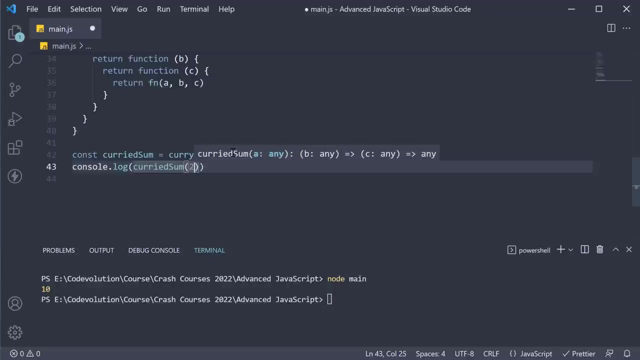 a, comma B, comma C. with this curry function in place we can now write const carried sum is equal to call the curry function passing in the sum function in the next line console log and we can invoke the curried sum function passing in one argument at a time. so curried sum of 2. 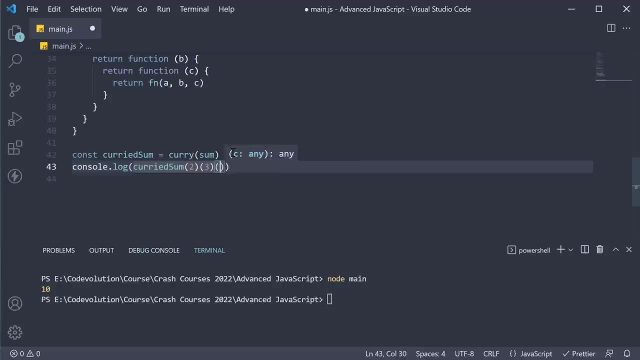 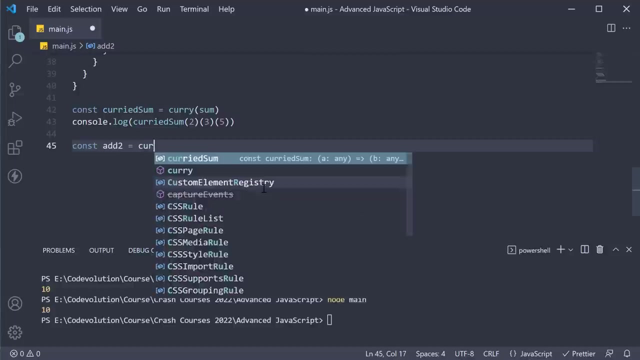 of 3 of 5 run node main and the output will still remain 10. now, if this syntax doesn't look that different from what you've been doing all this while, let me break this down. const add to is equal to courage- some we pass in to. const add 3 is equal to. 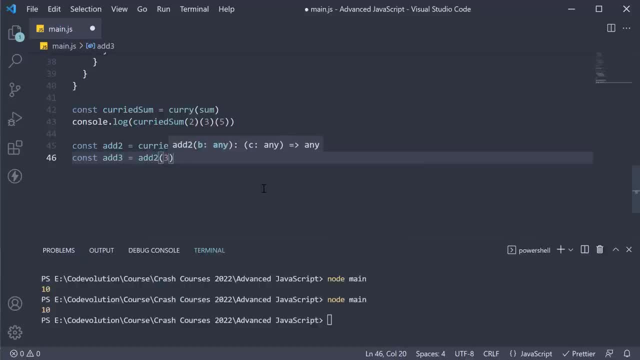 call add to passing in a value of 3, then const add 5 is equal to call add 3 passing in 5. finally, log to the console add 5. the three parentheses can be broken down into three separate function calls. the first function takes the first argument. second takes the second argument and. 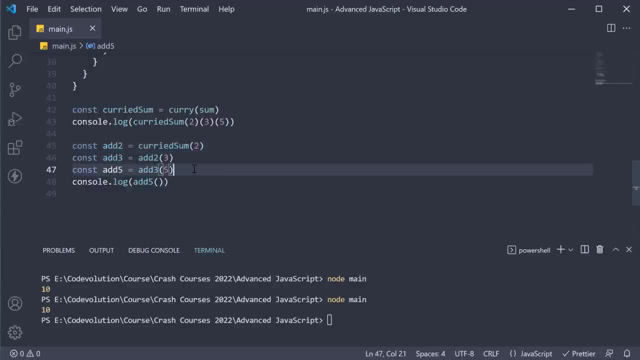 third, takes the third argument, then computes the sum of all the three arguments and returns the result. so this will just be add 5 instead of invoking add five, run node main and we see 10 from both the log statements. we have transformed a function with multiple arguments into a sequence of nesting functions that take one argument at a time. 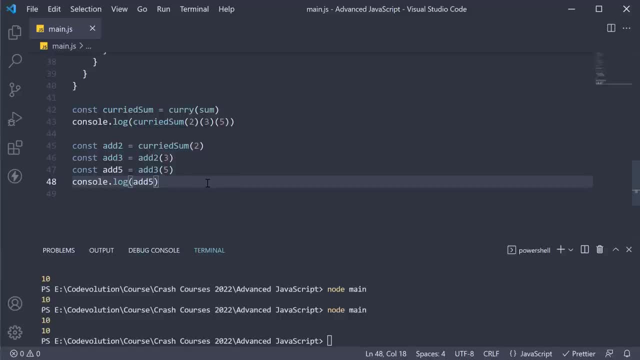 now, currying is used to compose reusable functions. for example, you can create functions like log info, log error, log now, etc. where one or more arguments are set and you get to choose the remaining arguments. currying makes composing new functions very easy. if you have understood the general concept about currying, i would recommend you take a detour. 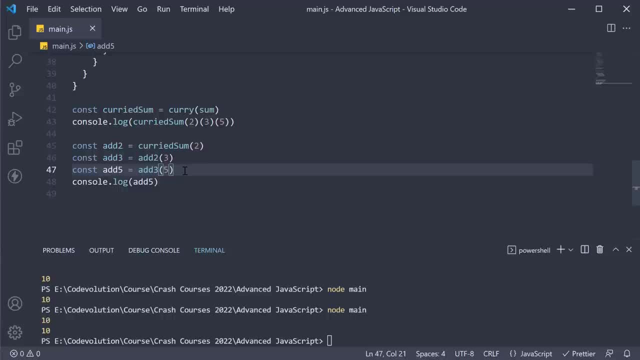 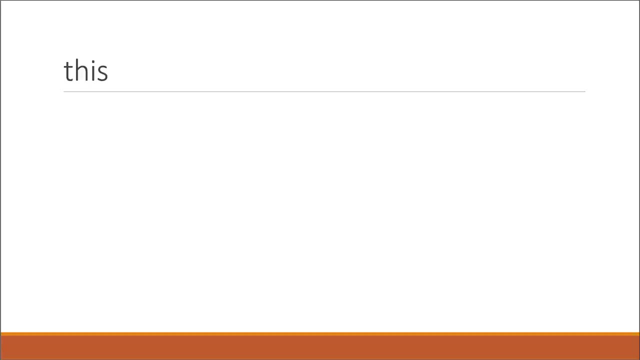 google more about function currying and get an understanding of the practical applications. all right, we are now going to move on to one of the most confusing parts of javascript, which is this keyword, the javascript. this keyword, which is used in a function, refers to the object it belongs to. it makes functions reusable by letting you decide the object value. 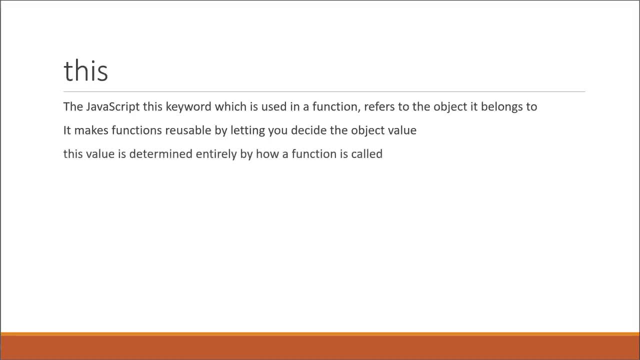 and this keyword value is determined entirely by how a function is called. now, if that doesn't make sense, let's understand how a function is called. so let's go back to our first example. let's now go back to our first example and see how we can use this function and also in this example. 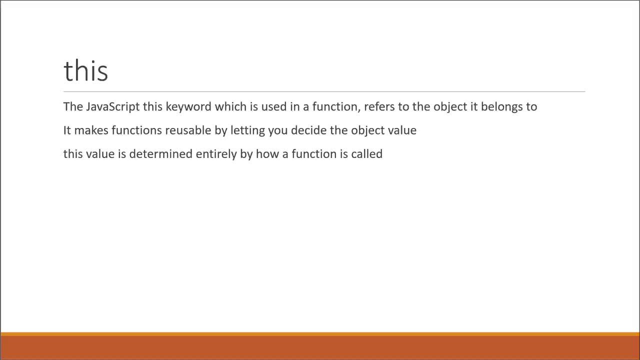 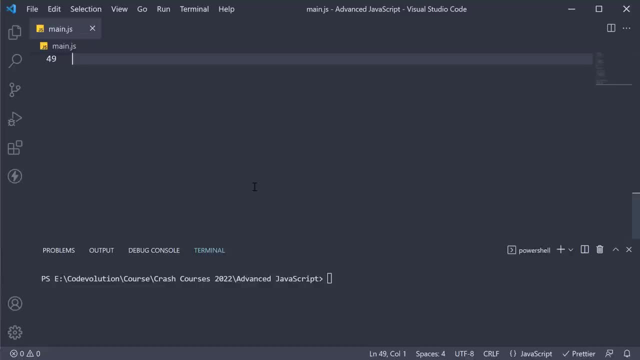 understand, with a few examples, how to use this keyword and how its value changes based on the function call Back in VS Code. let's define a function called sayMyName which has one parameter name and logs to the console. My name is followed by the name passed in. 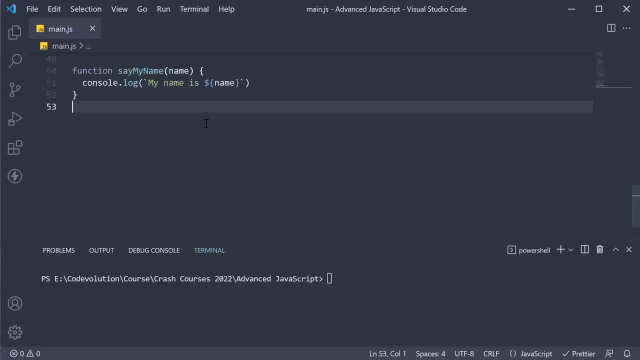 Looking at the function. if I were to ask you what would this function log to the console? you would say: we can only determine that looking at the function call. If I call the function passing in Walter White, you would say the output is hello, my name is Walter White. If I call the. 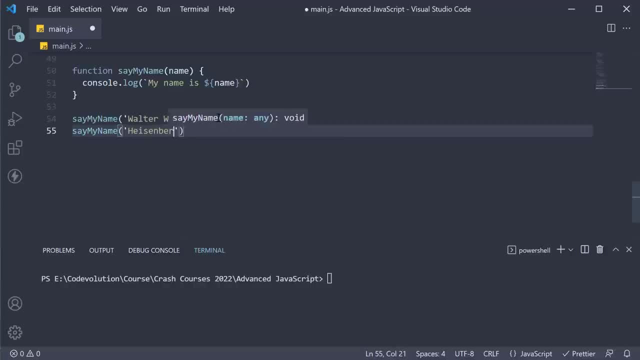 function passing in Heisenberg, you would say the output is hello, my name is Walter White. If I call the function passing in Heisenberg, you would say the output is hello, my name is Heisenberg. so you can determine what is logged to the console by: 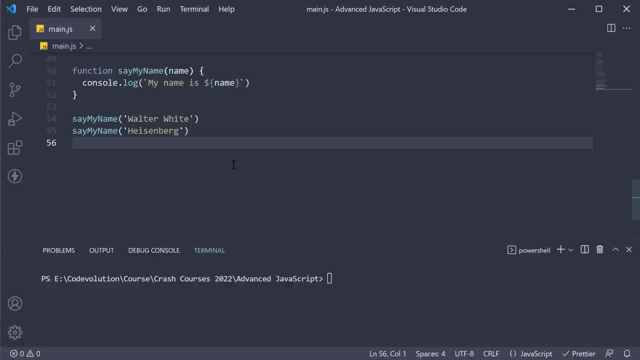 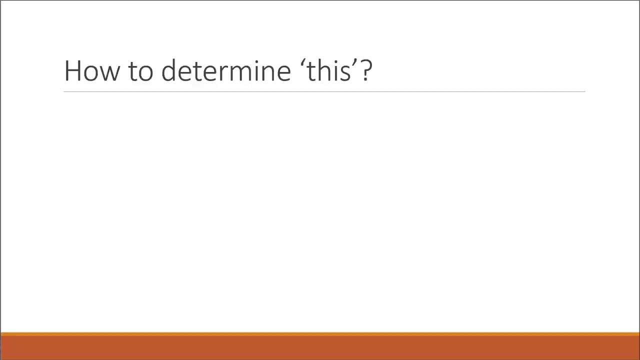 how a function is called, and this is the same with this keyword. you can determine the value of this keyword by how a function is called. now there are four ways to invoke a function in JavaScript and determine the value of this keyword: implicit binding, explicit binding, new binding and, finally, default binding. let's look at examples for each of them. first, implicit binding. 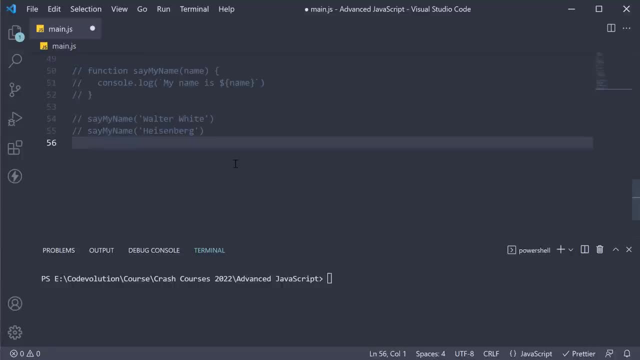 implicit binding rule will tell you what this refers to most of the time. consider an object. first of all, we need to define the value of the function in javascript and determine the value of the function with a property called name. set to wish was also a function or a method, to be more. 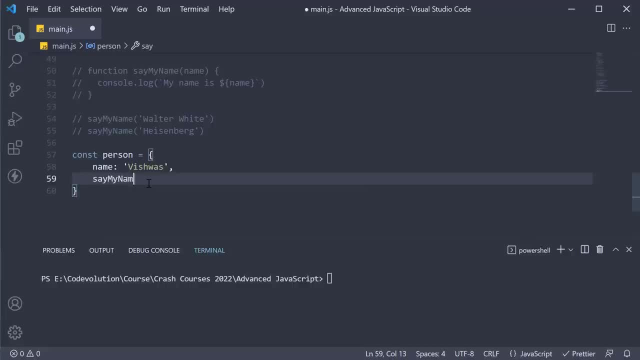 precise called, say my name, which logs this dot name to the console. my name is dollar curly braces and we evaluate this dot name to invoke the function in javascript and determine the value of the function we use. the dot notation is a person dot say my name. we now know how the 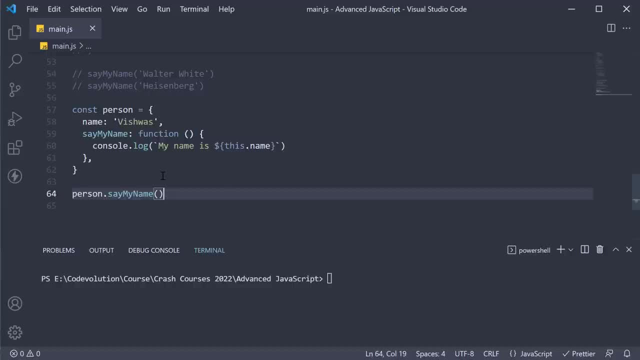 function is called, which means we now have what we want to determine this keyword inside the say my name function. the implicit binding rule states that when a function is invoked with the dot rotation, the object to the left of the dot is what this key membere isiders: a dot. 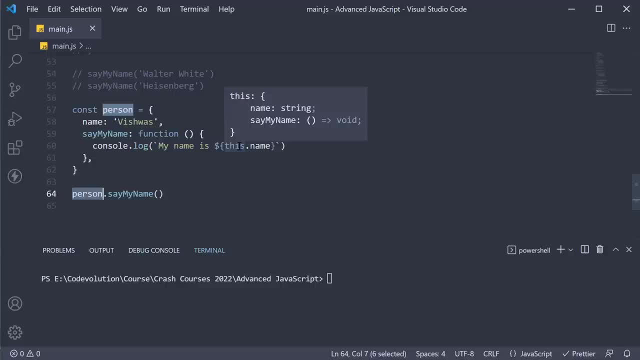 referencing javascript will now treat this dot name as person dot name, which is equal to the string vishwas, and the output, if i run node main is my name is vishwas. this is the implicit binding rule. the second rule to determine this keyword is explicit binding. consider the same function. 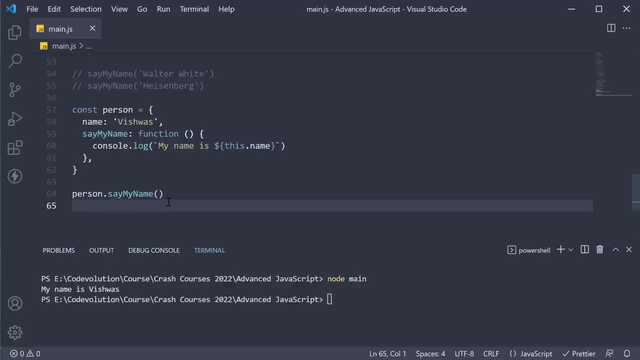 say my name, but this time the function is separated from the person object. so function say my name and we log to the console. my name is this dot name. in this scenario, we have to explicitly specify the context when the function is called. to do so, we can use the call method. 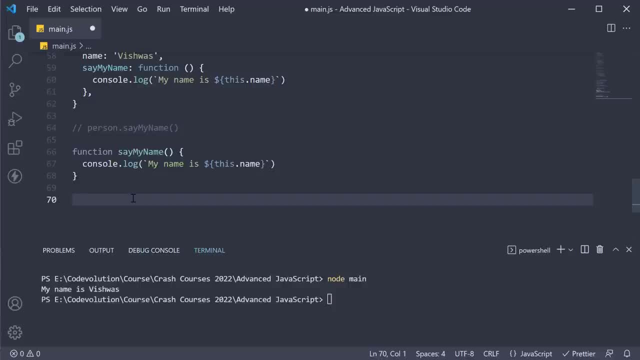 in JavaScript, every function has a built-in method named. you can use the call method. in javascript, every function has a built-in method named call, which allows you to specify the context with which a function is invoked. so to invoke, say my name, with the person object context, we have to write say my name dot call with person as the. 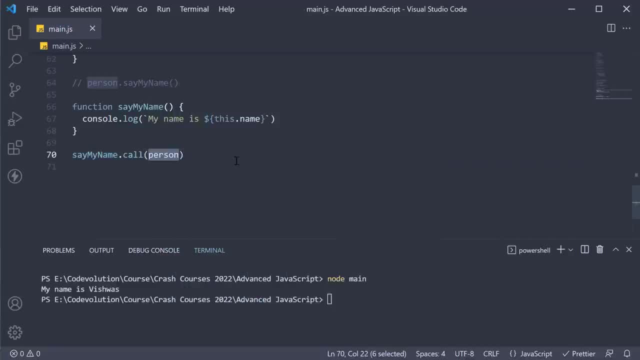 argument. the first argument passed to call is what this keyword inside say my name is referencing. if you run node main and you log to the console, my name is this dot name. in this scenario we have to set the next function, which is the key to the code. so if i run node main, the code will once again. 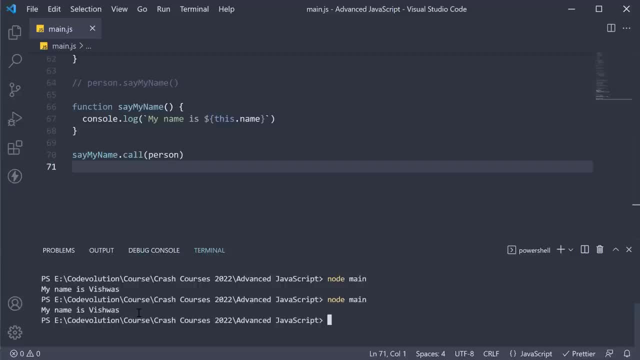 output. my name is vishwas to the terminal. so this is the second rule, which is explicit binding. the third rule for determining this in a function is the new binding in Javascript. we can invoke a function with the new keyword and in such a scenario, the function is invoked with this keyword. 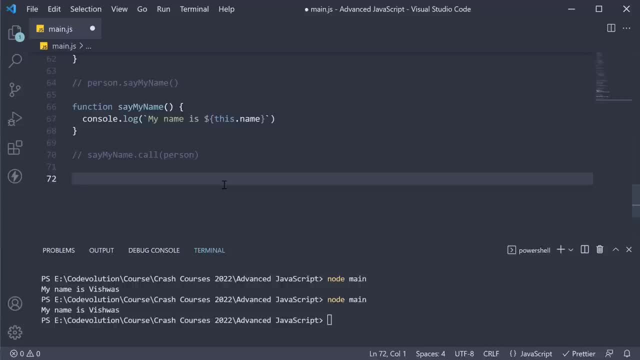 referencing an empty object. So consider a function called person which accepts a name Within the function we set, thisname is equal to the passed in name. With this function, we can now create multiple persons or people passing in different names each time. 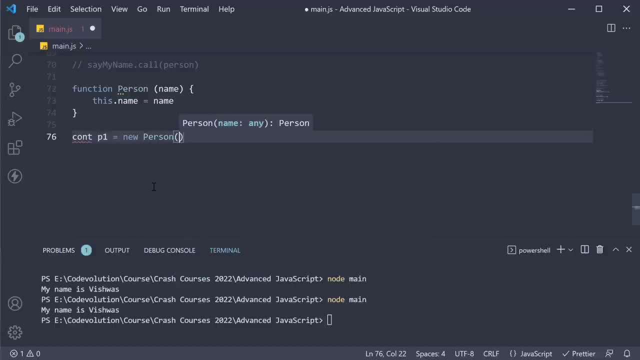 So const p1 is equal to new person and the name can be Vishwas, And similarly, const p2 is equal to new person we pass in Batman. This person function right here is what is known as a constructor function, as we can create multiple persons from this function. 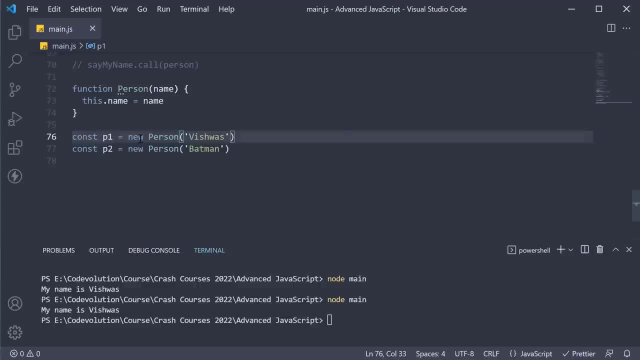 Now, when we invoke a function with this new keyword, JavaScript under the hood will create a new empty object That this keyword will reference. So within function person, I'm going to add as a comment: this is equal to an empty object. 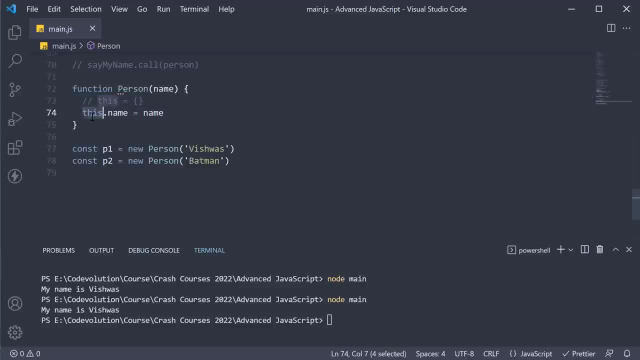 You can then add properties to the object using this, followed by the dot notation, So this dot name is equal to name. We are not creating this empty object. The new keyword internally. It does this when function person is invoked with the new keyword. 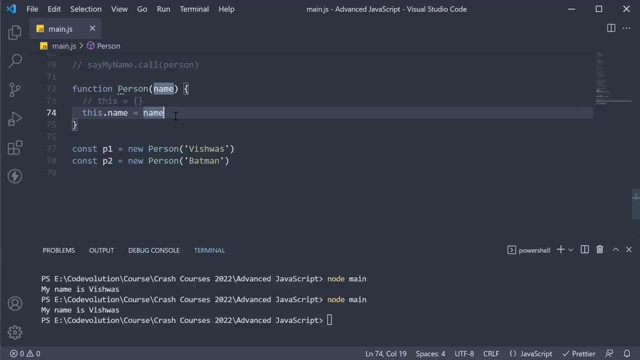 The new keyword also does a few other things, But from this keyword point of view, I just want you to remember the following line: When a function is invoked with the new keyword within the function, this keyword will always reference a new empty object. 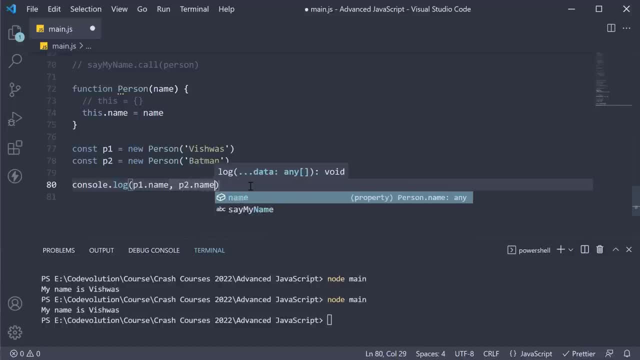 So if we log p1 dot name and p2 dot name Run node main, we see Vishwas and Batman in the terminal. All right, the fourth and final rule is the default binding, which is the fallback binding if none of the other three rules are matched. 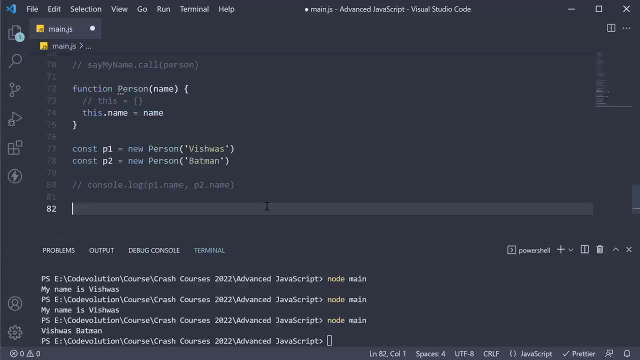 So consider the same say my name function. Let's call it as you would normally call a function: Say my name- with parentheses. As you can see, there is no dot notation, no call method or no new keyword as well. If we simply invoke say my name, what do you think the output is? 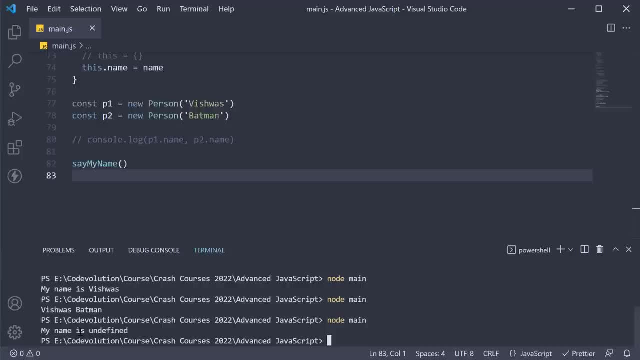 Run node main And you can see it is. my name is undefined. So if none of the three rules are satisfied, JavaScript will default to the global scope and set this keyword to the global object. In the global scope, JavaScript will try to find a variable called name. 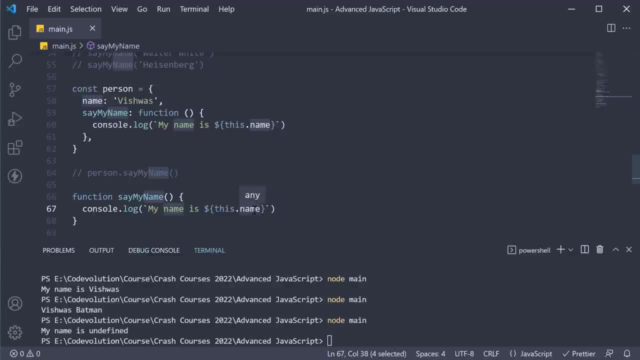 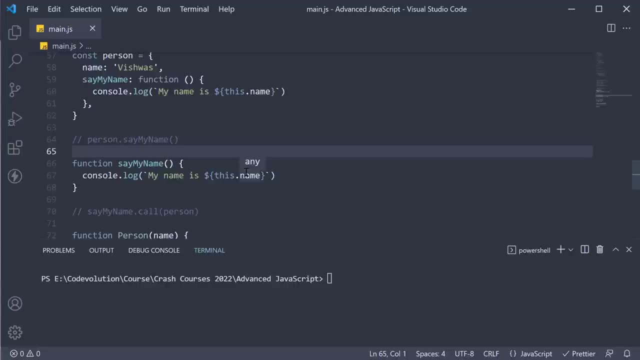 Since it doesn't find it, this dot name is undefined. If you were to have the variable name in the global scope, however, So const name is equal to superman if it were to be a browser, But since it is node global, this dot name is equal to superman. 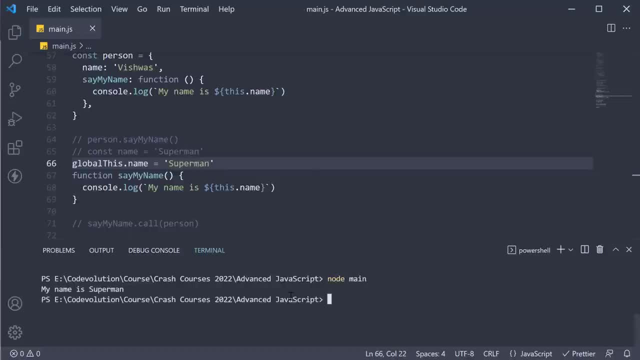 Run node main. You can see the output is: my name is superman. So the fourth binding is the default binding, where this keyword will rely on the global scope. As you can see, with this keyword you can introduce a dynamic value within the same function. 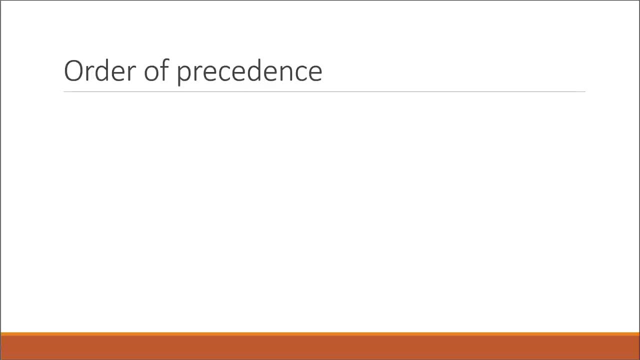 What you should know is that when multiple rules can be applied to figure out this keyword, new binding takes top priority, followed by explicit binding, followed by implicit binding, followed by default binding. So this is how this keyword works in JavaScript: It lets you specify the execution context, and its value is pretty much determined by how the function is invoked. 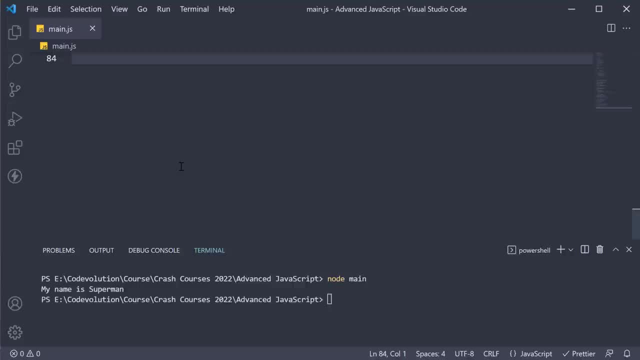 All right. Next, let's take a look at another concept. that is usually difficult, So let's take a look at the concept of prototype. When we try to understand everything, it may lead to confusion and us losing interest in the topic, especially as beginners. 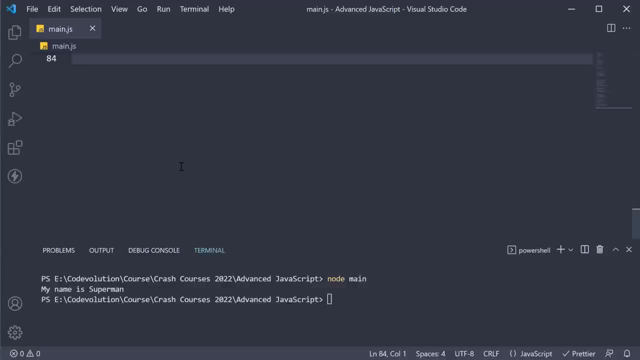 When it comes to prototype, there is a lot of terminology And when we try to understand everything, it may lead to confusion and us losing interest in the topic, especially as beginners. In this crash course, we will learn, with a simple example, why and how prototype works in JavaScript. 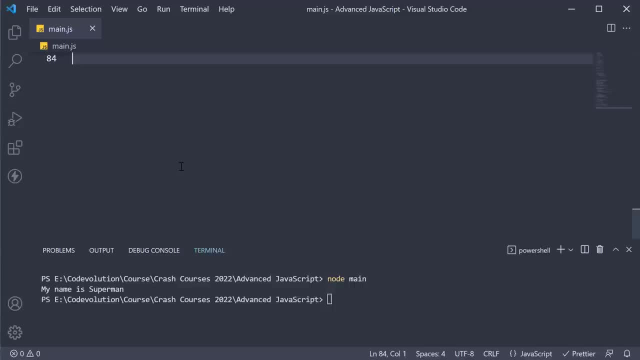 Let's begin by defining a function called person. So function person has two parameters, firstName and lastName, And within the function we're going to write, thisfirstName is equal to the past in firstName and thislastName is equal to the past in lastName. 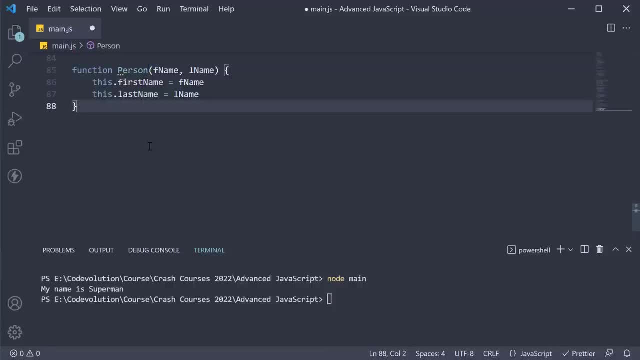 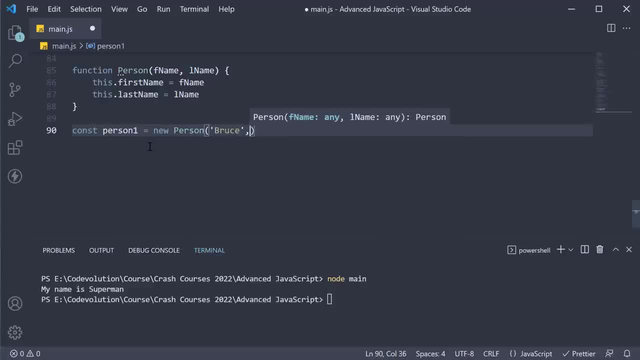 And we pass in Bruce Wayne. Similarly, const person2 is equal to new person, And we pass in Clark and Kent. Now, as you already know, JavaScript is a dynamic language, So it allows us to attach new properties to it. 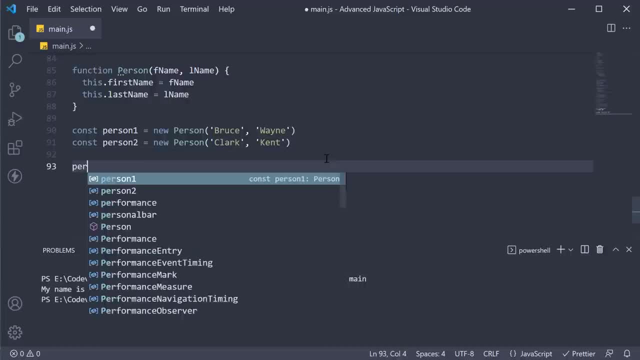 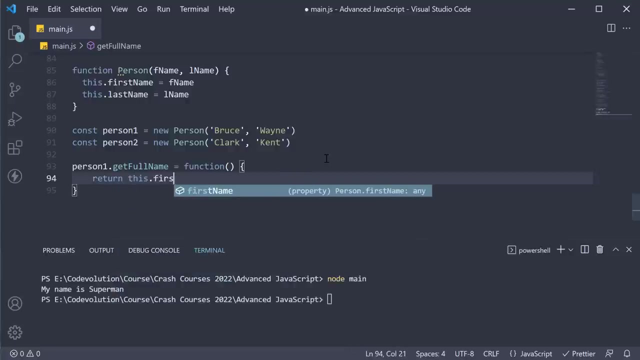 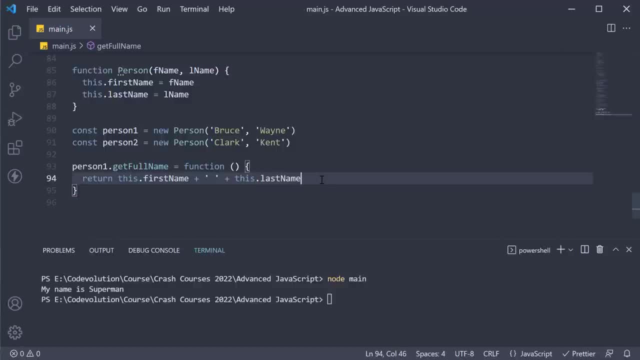 You can also use the template literal syntax for string concatenation. Now, what you should know here is that getFullName property is specific to just person1.. If we log person1.getFullName to the console, run node main, we see Bruce Wayne logged in the terminal. However, if we run person2.getFullName, 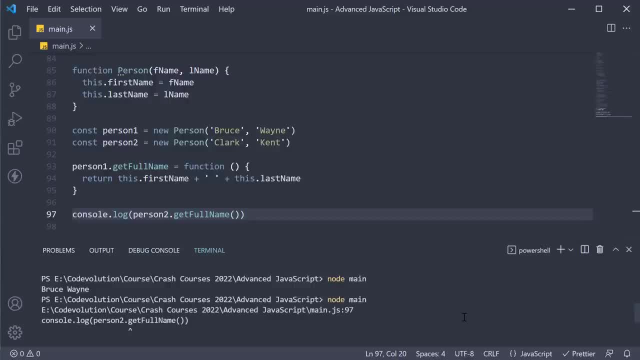 and run node main, we get an error. persongetFullName is not a function. Now what if we wanted to attach a property or a method that should be applied to every instance of this person function? In our example, getFullName is a function that benefits us by. 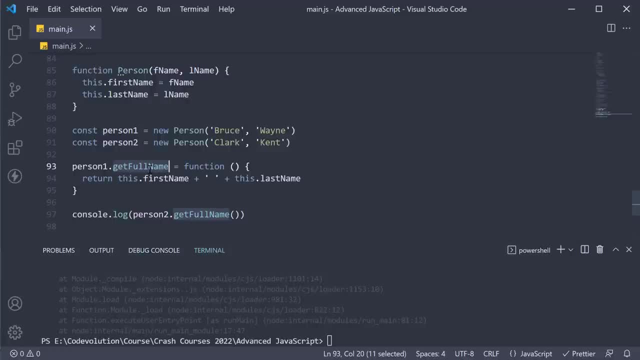 being available on all instances of the person function. since it is generic, It is not specific to just person1.. It would work on person1,, 2, 3 or even person100.. Well, this is where prototype comes into picture. In JavaScript, every function has a property called prototype. 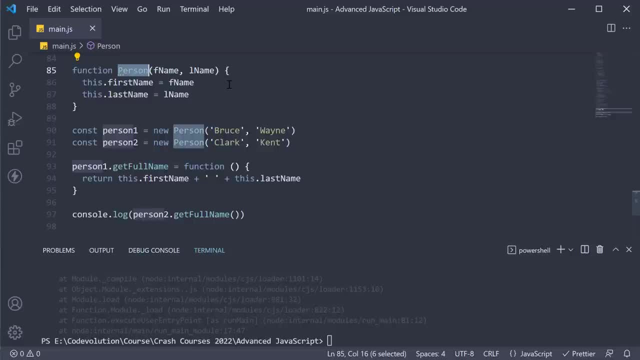 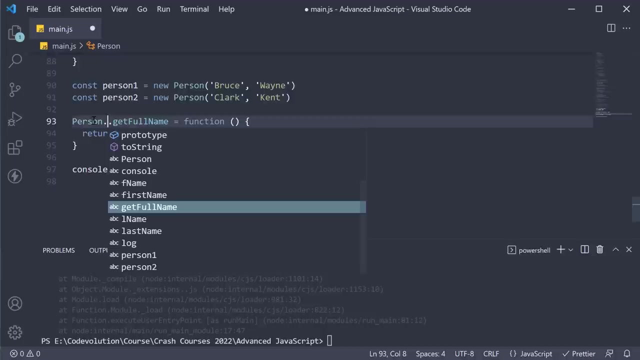 that points to an object. We can make use of that prototype object to determine all our shareable properties. So instead of person1.getFullName we change it to the person functionprototypegetFullName. Now if we log person1.getFullName and person2.getFullName run node main. we see Bruce Wayne and Clark. 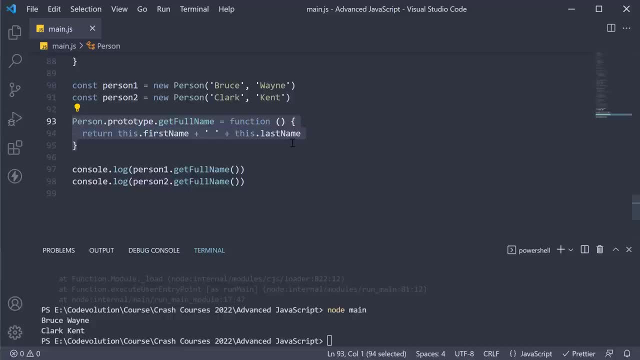 Kent. in the terminal We have defined the getFullName function. once Now if we log person1.getFullName and person2.getFullName, we find that have been used in a few instances ever on every instance of the person function. Again on a side note, the function that used with the new 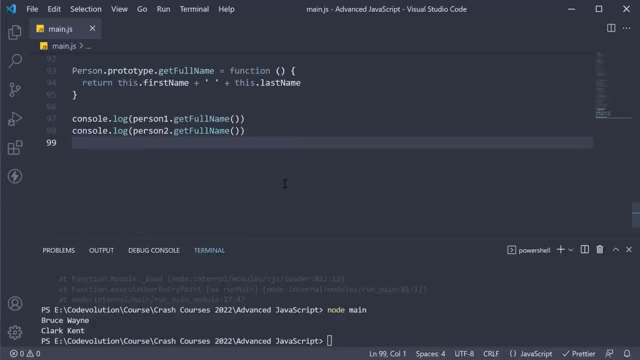 keyword is called a constructor function. Now, one use of prototype is to share properties and methods across instances. The other use, which is pretty significant as well, is inheritance. In JavaScript, inheritance is supported for a time if there is also a target value. instead, on the surre, Play沒事. 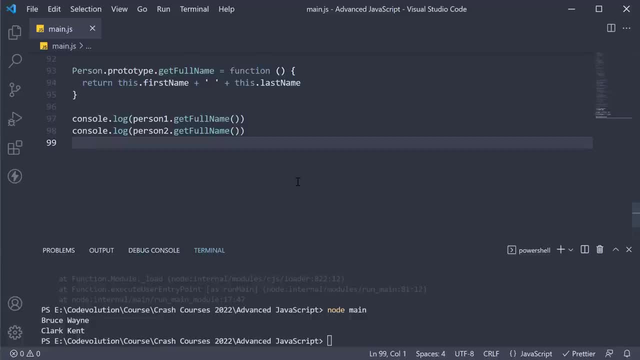 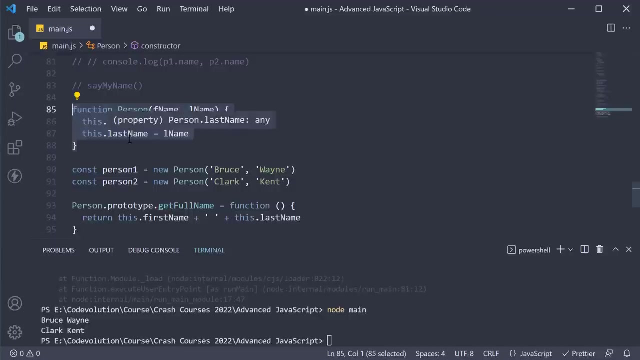 it to the concept of prototypes and is referred to as prototypal inheritance. Let's understand how it works. For our example. we're going to create a superhero that is supposed to inherit properties and methods from person, So a superhero will have a first name, last name and a getFullName function, but 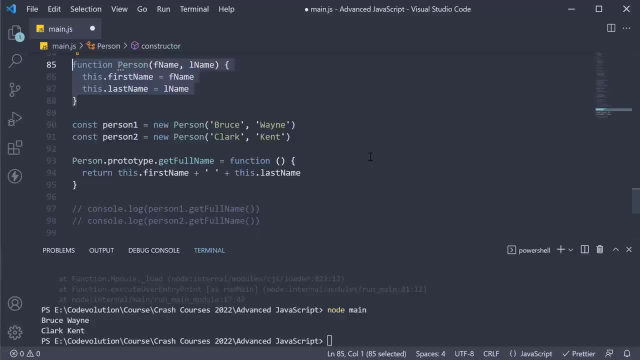 apart from that, a superhero will also have a property called easeSuperhero set to true, and a fightCrime function that logs a message to the console. Let me walk you through the code. Just going to rearrange the code. so there is continuity, and now we're going to begin by defining the superhero function. 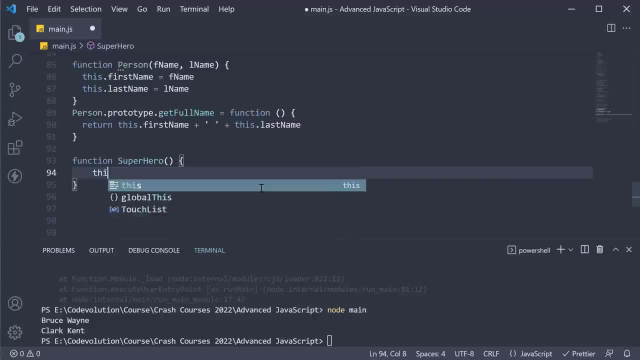 function superhero. We add one property called easeSuperhero and we set it to true. We also define the fight crime function on the prototype. So superheroprototypefightcrime is going to be equal to a function where we log to the console fighting crime. 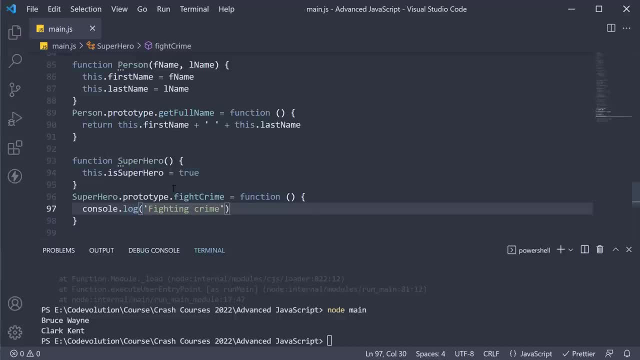 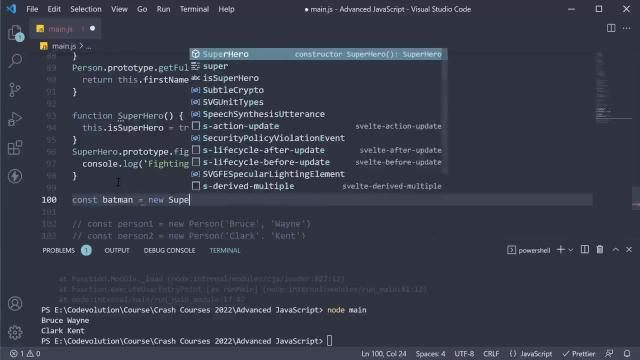 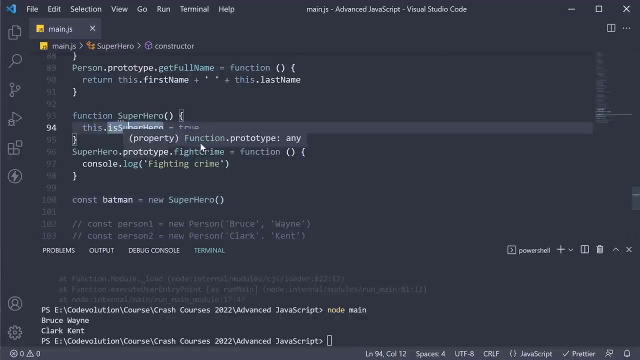 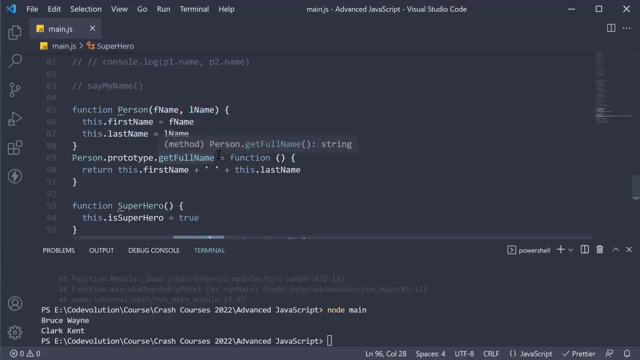 We can now create, just maybe a disclosure, create an instance of this superhero function. const batman is equal to new superhero. however, Batman only has access to ease superhero and fight crime. we want Batman to also have a first name, a last name and the get full name function. 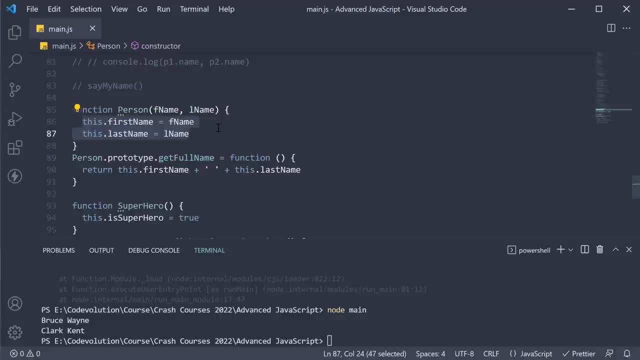 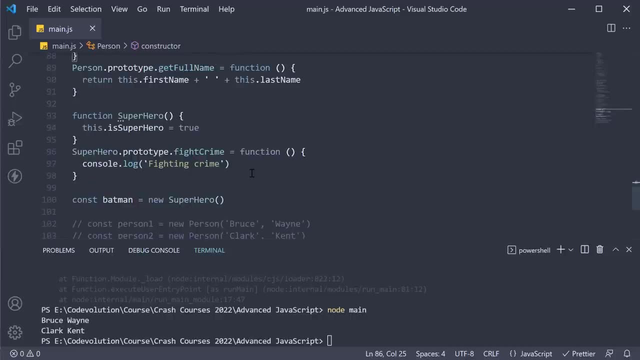 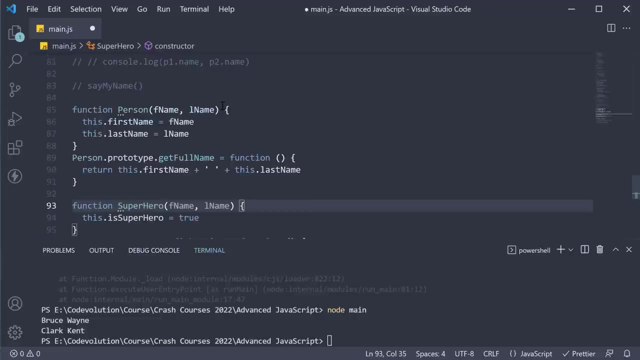 instead of duplicating the code we have written for person, let's inherit them first. let's inherit the first name and last name properties. superhero function will now accept two parameters: F name and L name. these values, though, need to be passed into the person function, but the person 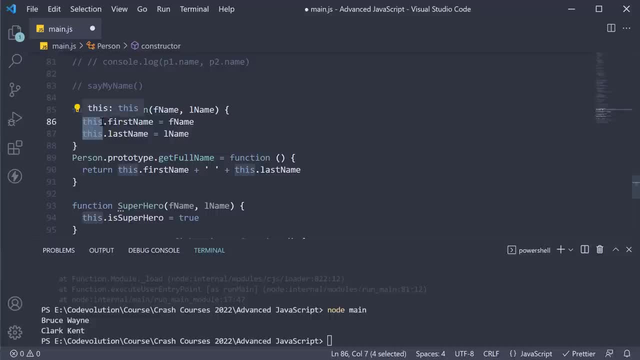 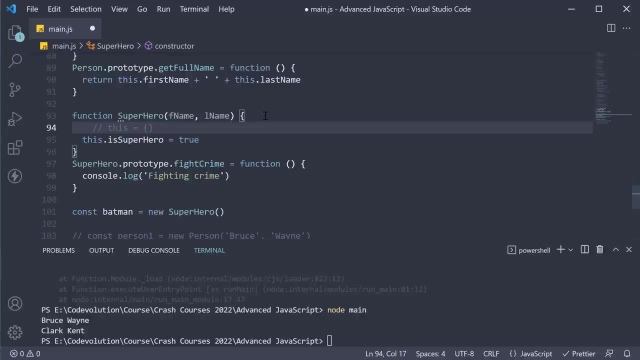 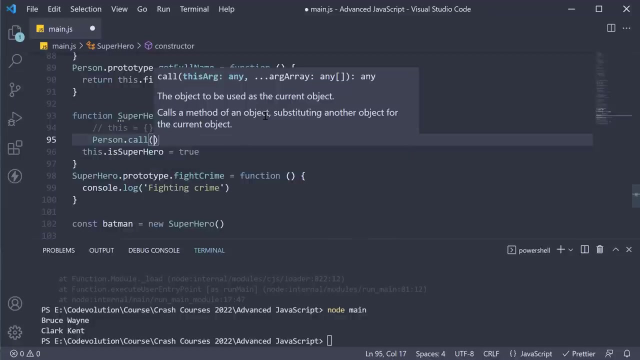 function should be invoked with this keyword pointing to this object from superhero function. and if you remember from the section on this keyword, we can call a function by specifying what this keyword should point to, using the call method. so person dot call and we pass in this keyword which is created inside the superhero. 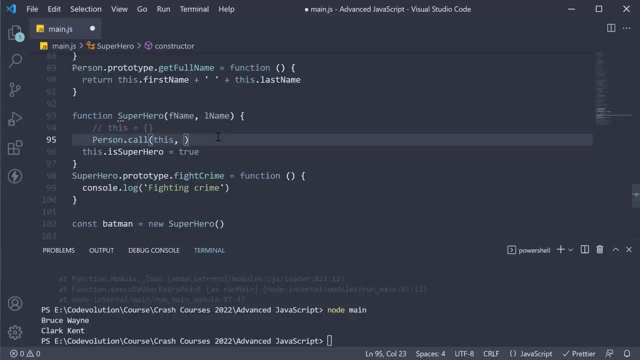 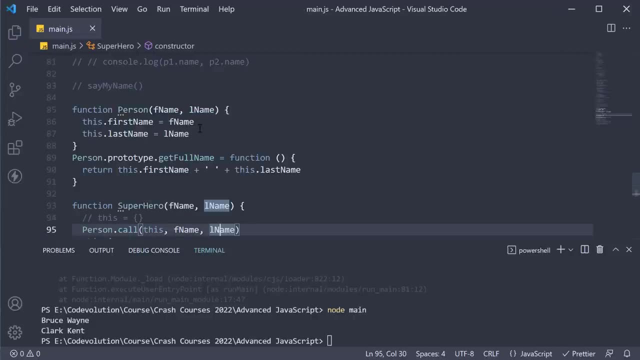 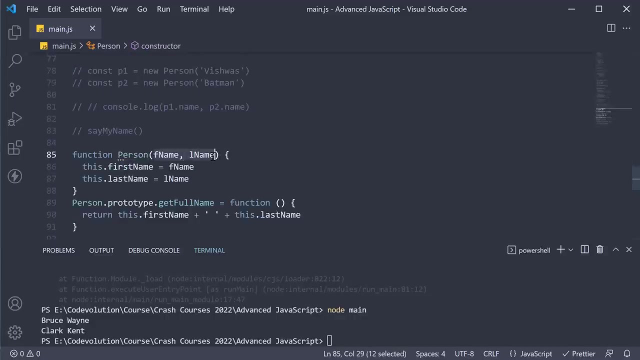 function as its first argument. second argument will be fname, third argument will be lname. so this keyword in person will now refer to this keyword in superhero. fname and lname get assigned and firstDame and lastName properties are now inherited by superhero. now to inherit the get full name method, we're 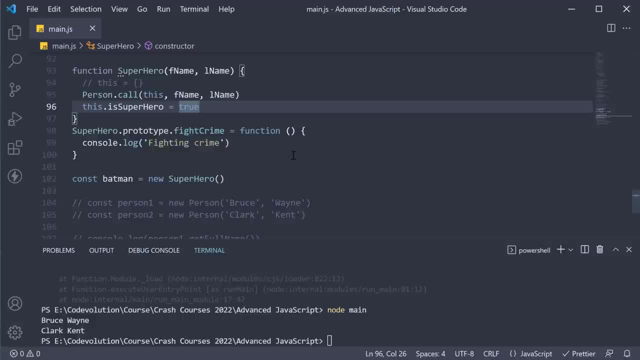 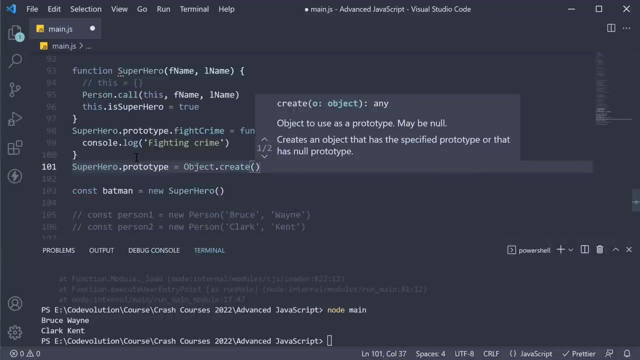 going to use objectcreate toograflex form, we go ahead and essentially use image type struct车, which is a method that will delegate to another object on failed lookups. So superheroprototype is equal to objectcreate and we pass in personprototype. 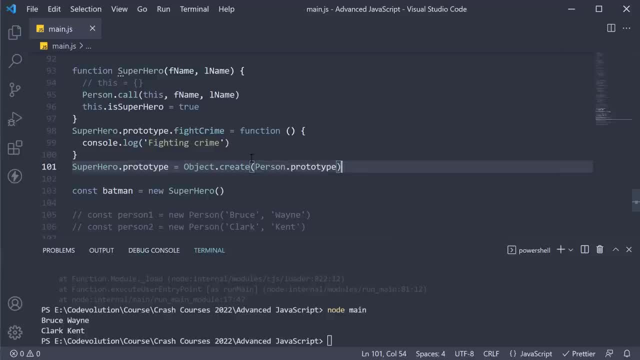 So what this does is when you try to access batmangetFullName, JavaScript checks the prototype object of superhero. It doesn't find it. However, it sees that the prototype object has a chain to personprototypeCreated because of this objectcreate method. 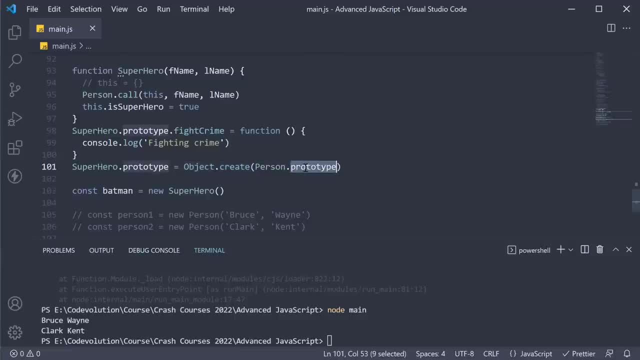 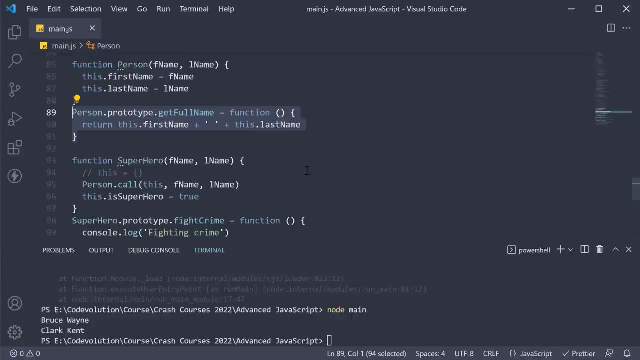 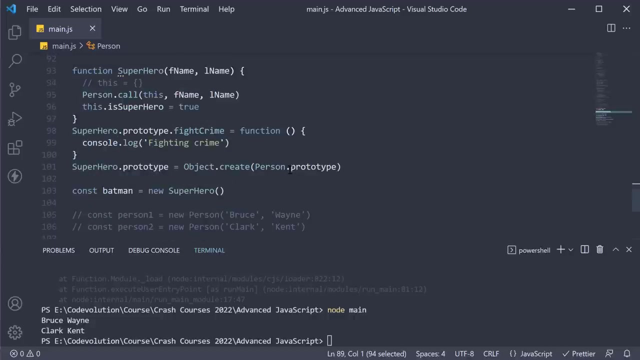 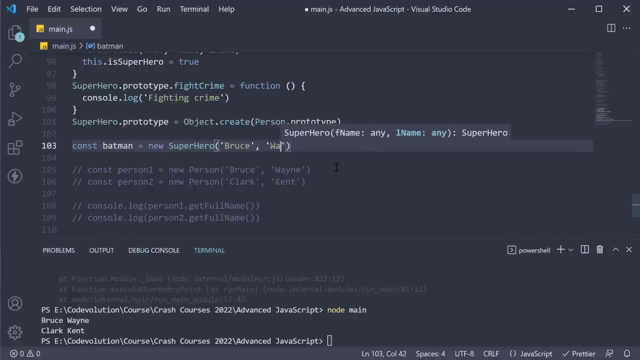 It checks to see if personprototype has a getFullName method. It does, and it will execute that method. This is how the method is inherited through the prototype chain, Hence the nameprototypalinheritance. So if we now pass in Bruce and Wayne while creating batman, 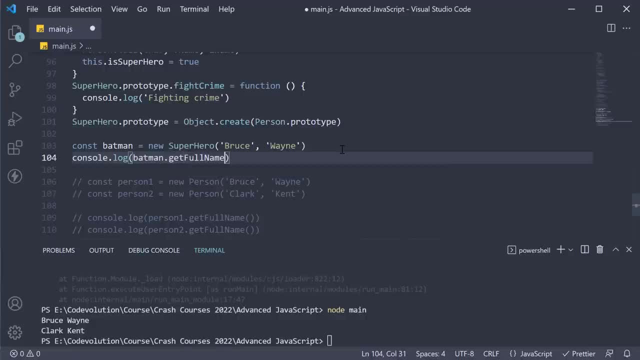 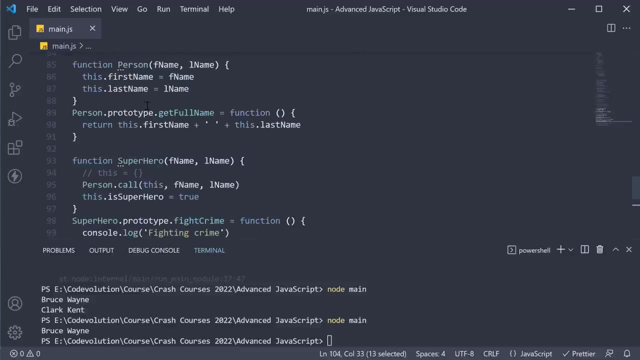 and log batmangetFullName run node main and we see Bruce Wayne logged in the terminal. Batman superhero has inherited getFullName from getFullNameinheritance. The method will access thisfirstName and thislastName, which are also inherited by the superhero function. 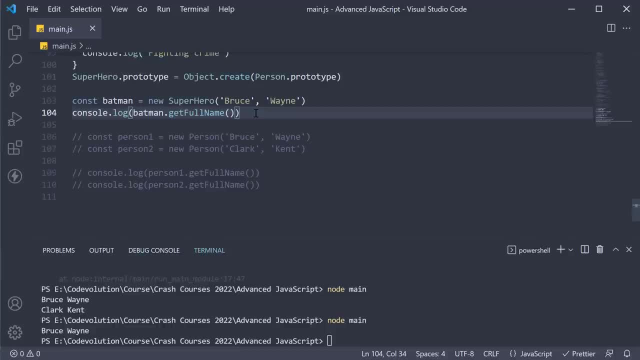 Now, one last bit of cleanup we need to do is to ensure superheroprototypeconstructor is equal to superhero. Otherwise, JavaScript thinks that a superhero is created from personprototypeconstructor, which is incorrect. Run the code again and we still see Bruce Wayne. 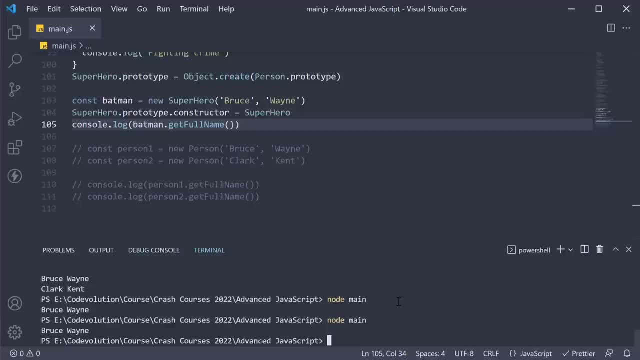 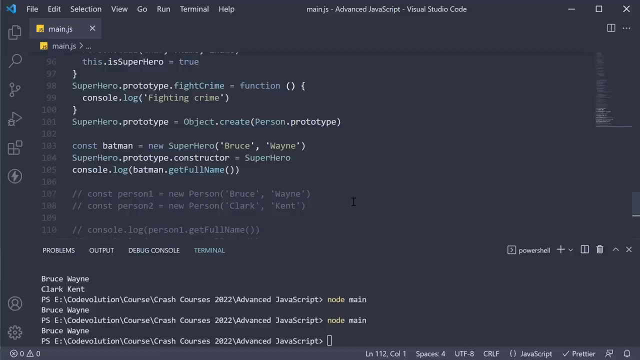 Superhero has inherited properties and methods from person. All right, for our next topic. we're going to learn about the class keyword, which was introduced in 2015.. A minute ago, we learned about prototypal inheritance. If you're coming to JavaScript from a language like 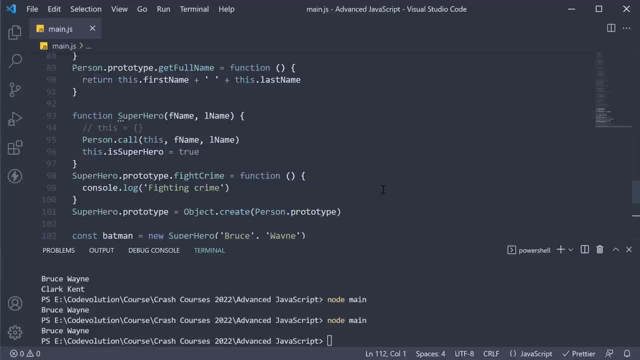 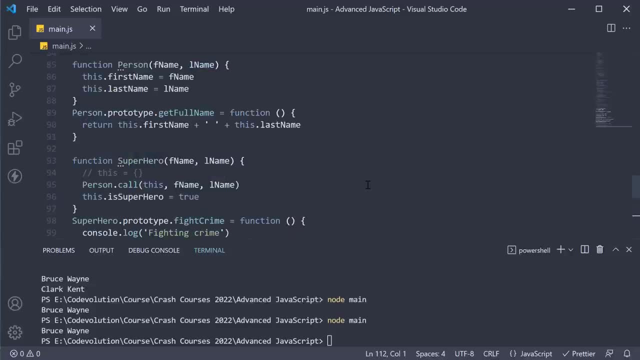 C++ or Java. it might be very confusing. You would be more used to class-based inheritance. Well, to somewhat relate to that, classes were introduced in 2015.. However, the class syntax does not introduce a new object-oriented inheritance model. 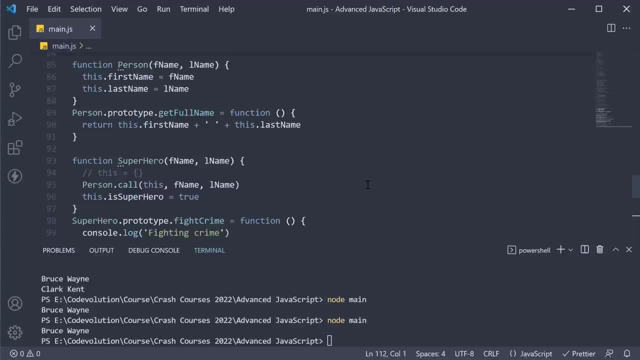 In JavaScript, classes are primarily syntactical sugar over the existing prototypal inheritance. In JavaScript, classes are primarily syntactical sugar over the existing prototypal inheritance. Let's learn how it works by rewriting the prototypal inheritance code with classes. 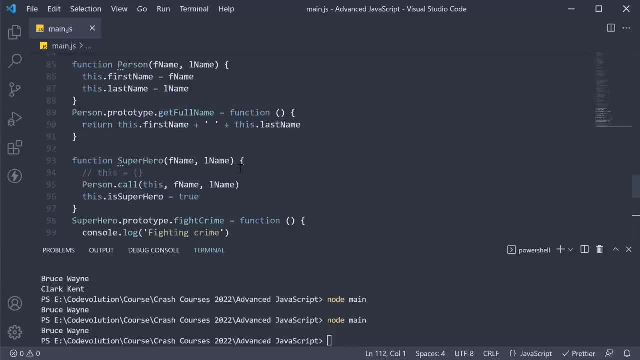 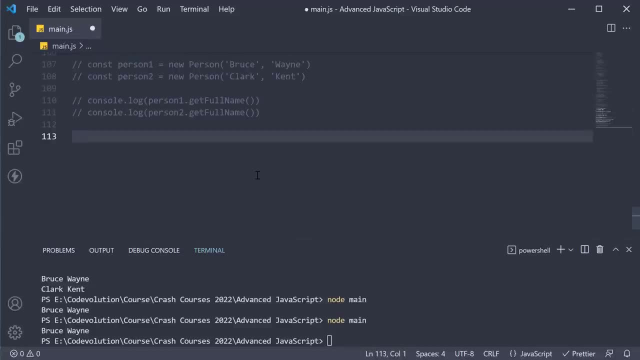 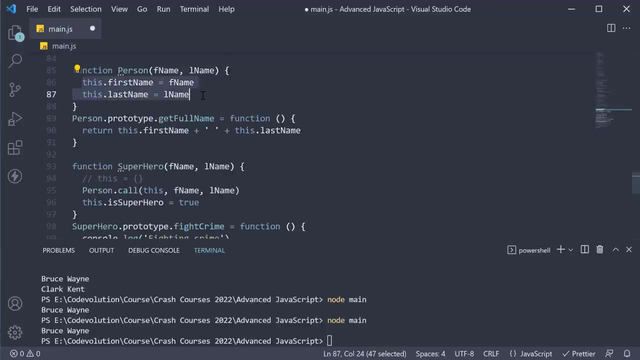 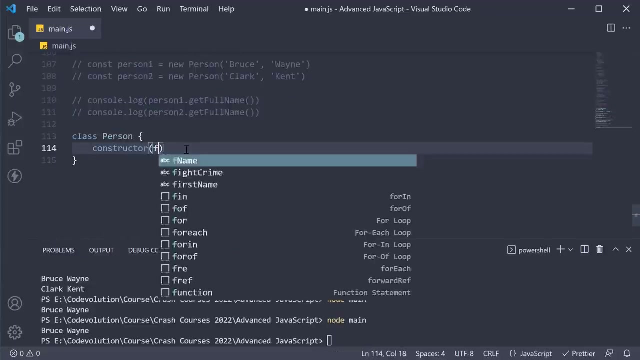 Let's learn how it works by rewriting the prototypal inheritance code with classes. Let's start with this person function. First change: function: person becomes class person. The initialization of the name argument to this object gets moved into a constructor. So constructor accepts first name and last name. 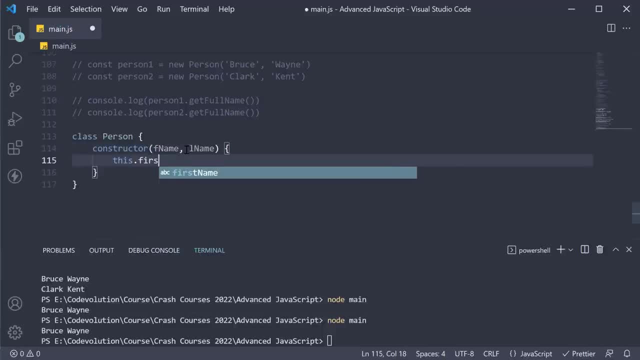 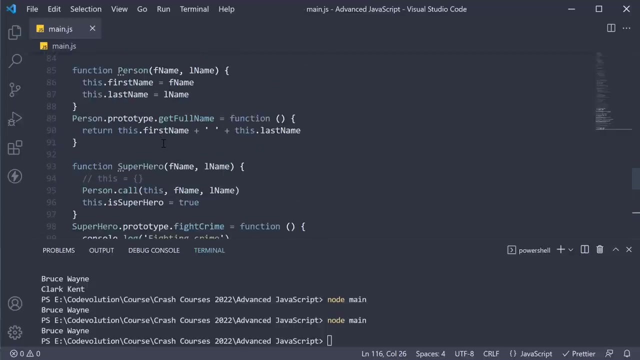 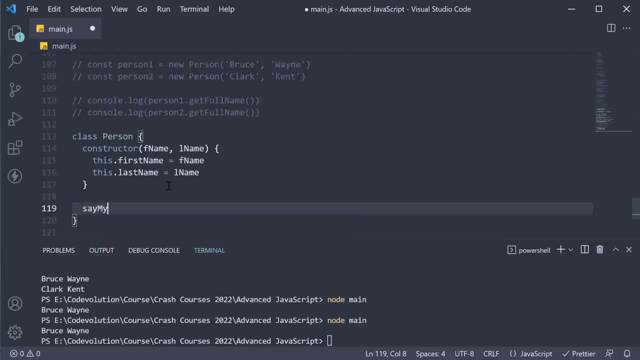 name and within the constructor, this dot first name is equal to F name. this dot last name is equal to L name. second and final change: all the methods on the prototype object are rewritten as methods within the class. so say, my name is a function where we return. 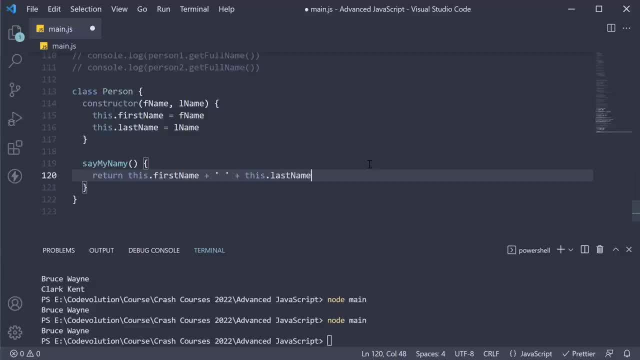 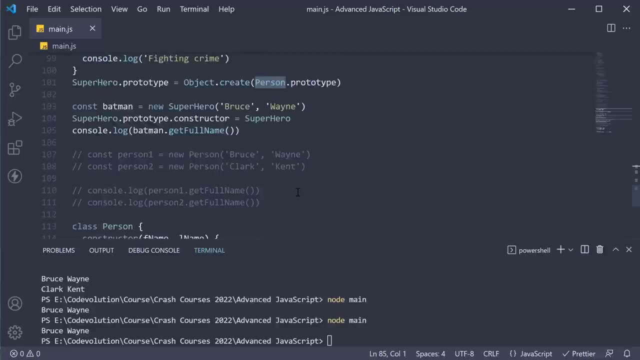 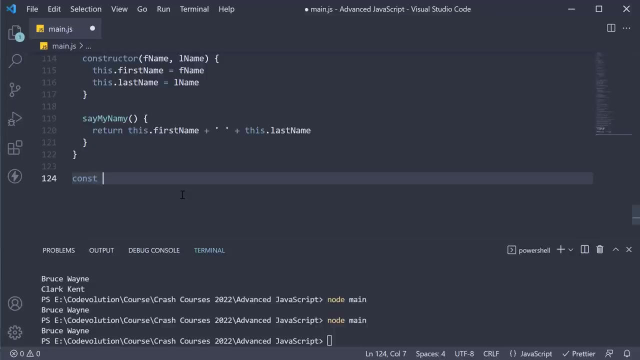 this dot first name, followed by this dot last name. it is as simple as that. we can now comment out the previous code and create instances of this person. so const class person one is equal to new person and we pass in Bruce and Wayne as arguments. we can now log class p1. 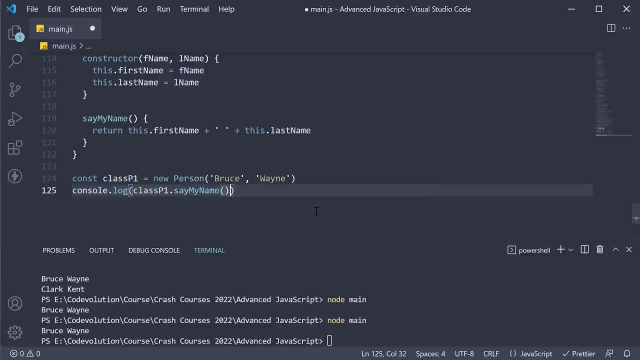 dot. say my name to the terminal and we see Bruce Wayne being logged, So we can create an instance and access the properties and methods like before. Nothing changes. The class keyword simply makes the syntax better for the code we already had in place. Let's now rewrite superhero, which. 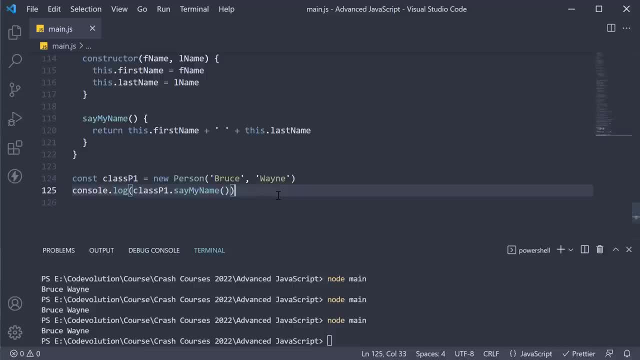 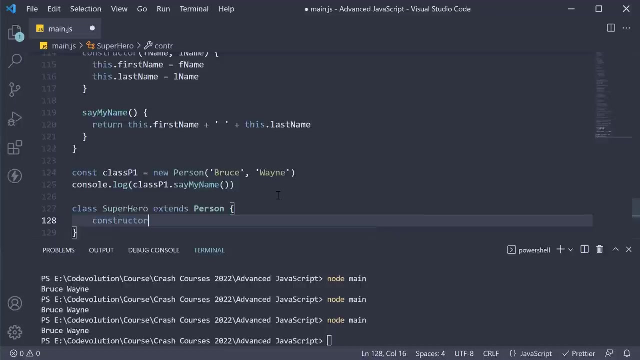 inherits from person, Two keywords take care of the entire inheritance and those two keywords are extends and super. We specify that class superhero extends class person and in the constructor we accept first name and last name and we invoke the super method that JavaScript provides us passing in fName. 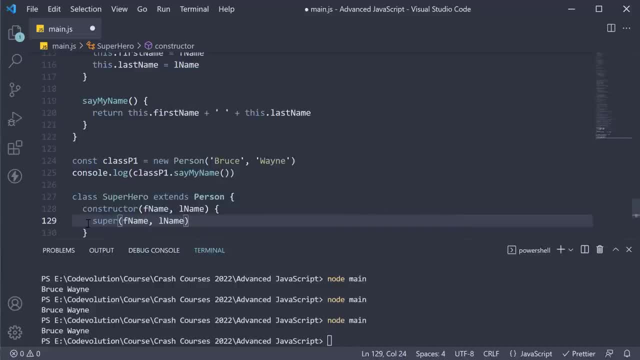 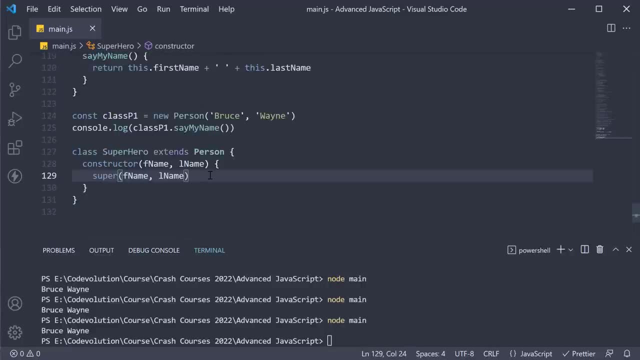 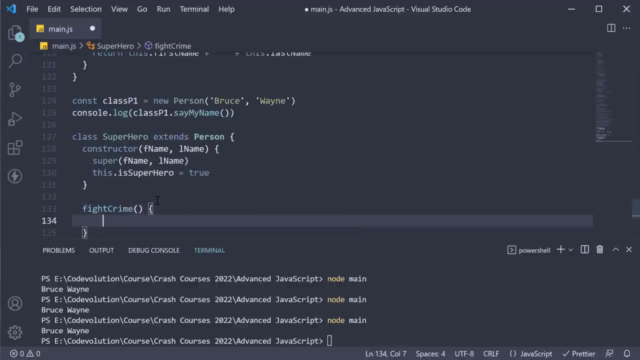 and lName. This will call the person class constructor. Once we call super, we set the superhero properties and methods in the class. This dot isSuperhero is equal to true. And then we define the fight crime method: Console dot log: fighting crime. 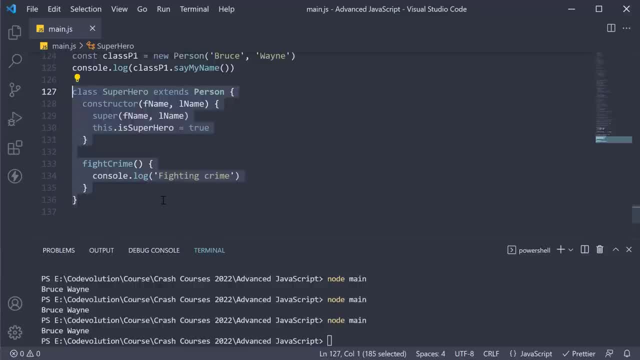 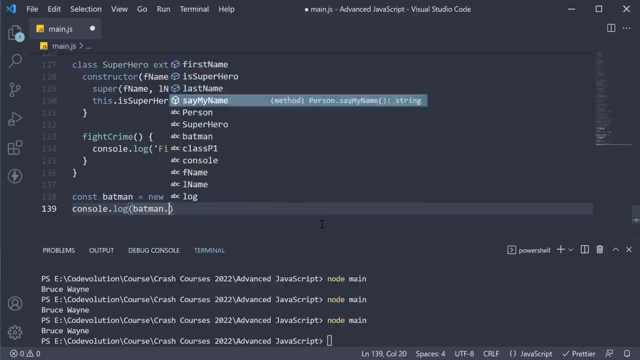 But this simple class syntax pretty much is all we have to write. Let me now create a new instance. So const Batman is equal to new superhero passing in Bruce and Wayne and we log Batman dot. say my name, Which we will print Bruce Wayne. 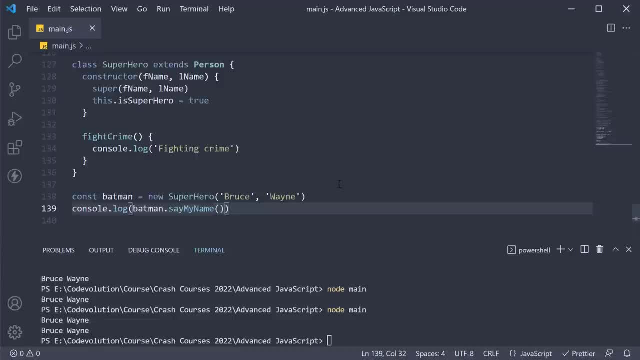 Again, let me reiterate: classes are just syntactical over what was already existing in JavaScript. Make sure you understand how to create a class, how to initialize properties, how to add methods, how to create an instance of the class, how to inherits using the extends and super keywords. 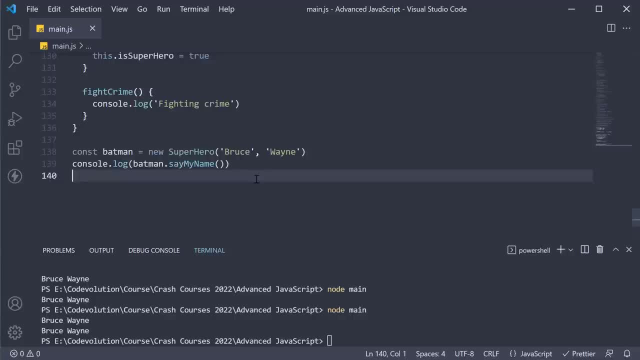 How to add methods, how to create an instance of the class, how to inherit using the extends and super keywords. that's all we have to say. That is pretty much all you have to know about the class keyword from a beginner's point of view. 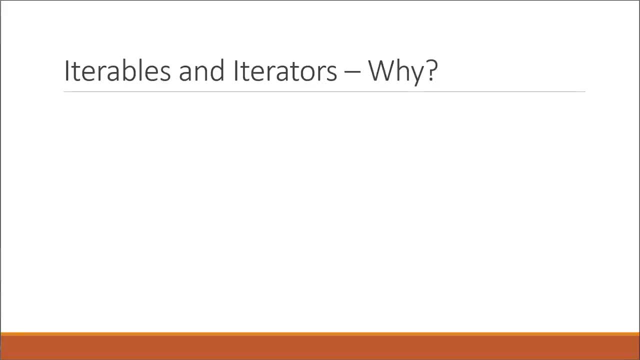 All right, let's move on to the penultimate topic in this crash course, which is iterables and iterators. I'm going to begin by setting some context about iteration in JavaScript. Before 2015,, we had three looping constructs for: loop, while loop and do while loop. 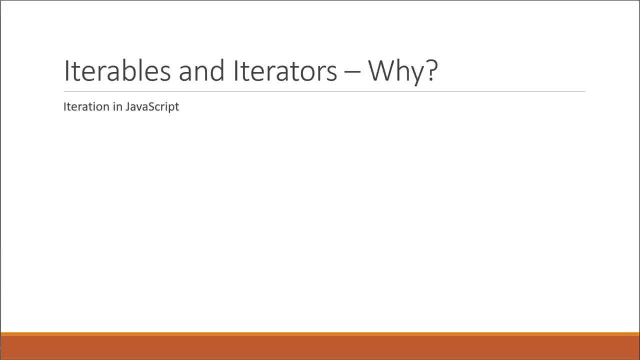 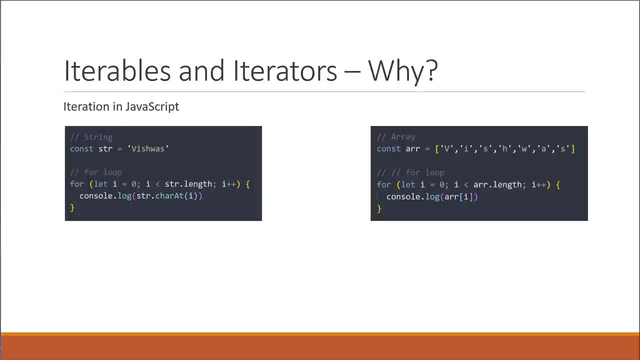 Let me show an example of how to iterate and access data with a string and array type using the for loop. On the left-hand side, you can see that we have stored the string Vishwas in a variable called str and we basically want to log every character in the string to the console. 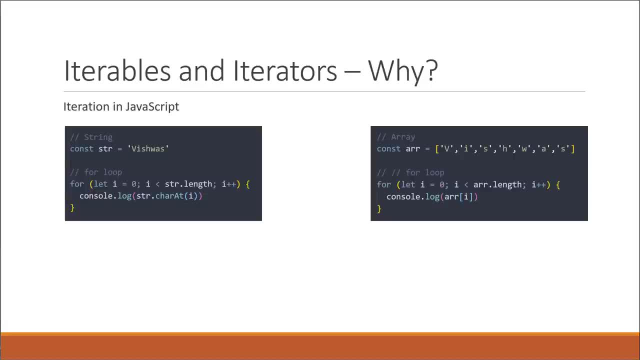 Similarly, on the right-hand side, the array is a collection of items which is nothing but the characters of the string we have already seen. We again want to log to the console each item in the array. Now this form of iteration has two difficulties, if I can call it that. 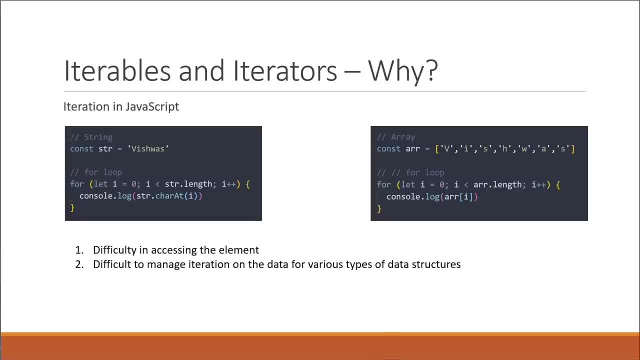 First to apply some functionality on each element in the string or each item in the array. we first need to figure out how to do that. We need to create a new variable i keep track of it, ensure it satisfies a condition and finally increment that value of i to access the next element in the collection. 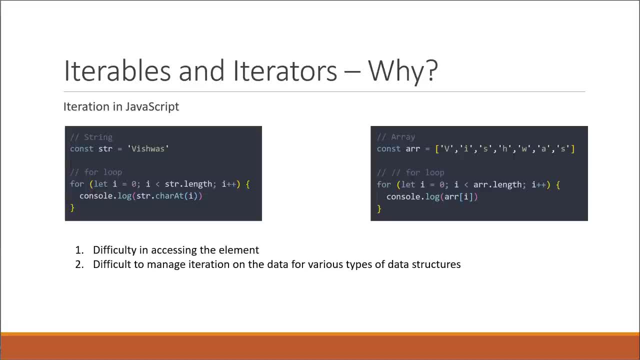 If there are nested for loops, we have to do this all over again with a second variable. So we would have difficulty in accessing the element itself before even getting to the part where we do something with that element. The second difficulty is with the type of the data structure. 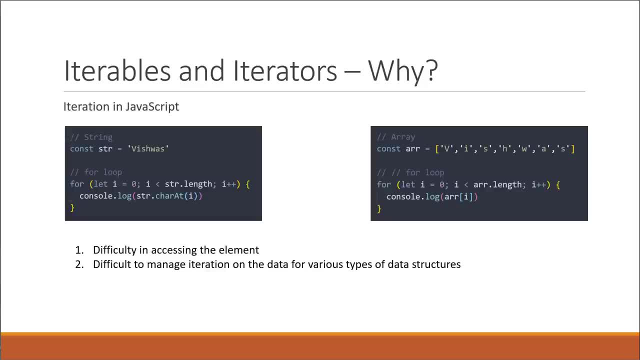 It is kind of difficult to manage iteration on data for various types of data structures. You can see that iterating and accessing elements on a string is different from iterating on an array, So there was a need to iterate over various data structures in a new way. 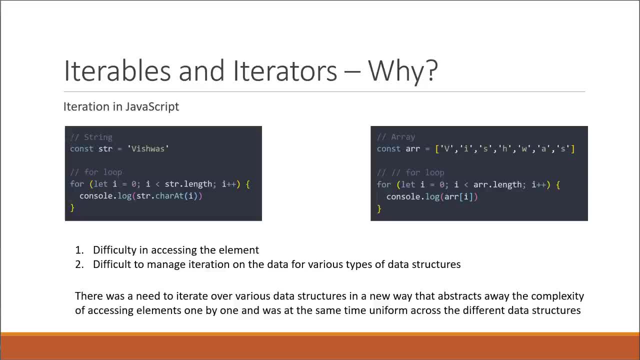 that abstracts away the complexity of accessing elements, so that the data structure remains one by one and was, at the same time, uniform across the different data structures. This would make our code more readable and less confusing. That is exactly the reason for the introduction of iterables and iterators in JavaScript. 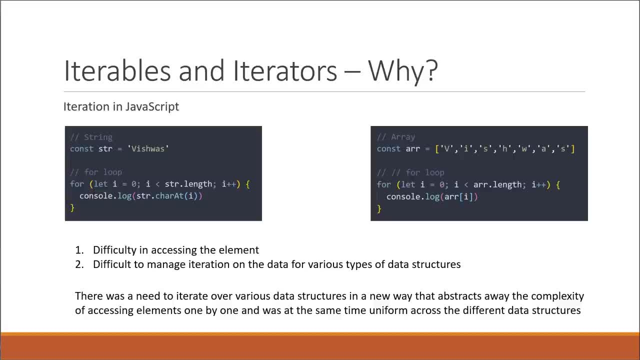 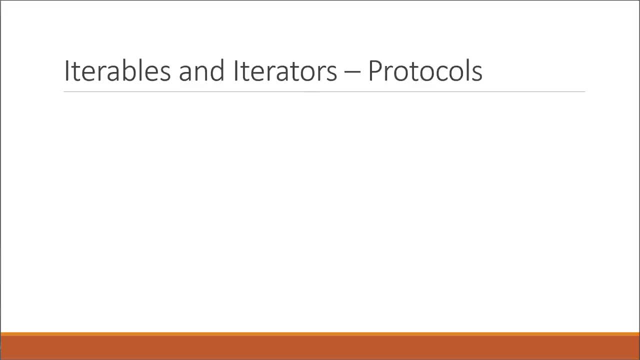 So let's take a look at how to do that. So this is the whrif repair device that we have been using In the year 2015,. two new Colorado scheduling protocols were introduced which help with iteration. they are the iterable and iterator protocols. 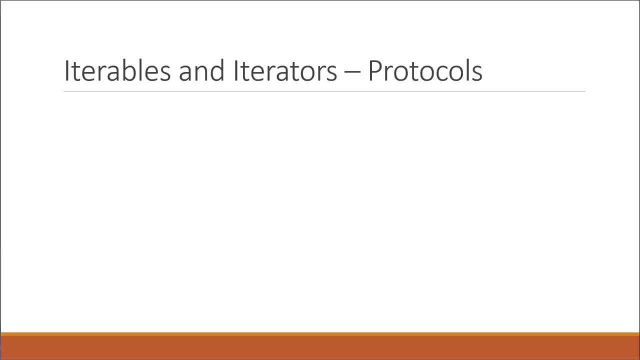 It was also decided that some of the data structures would implement the iterability protocol by default, The" which were dumping multiple iterations on different durations. Examples include strings, arrays and two more data structures which we haven't discussed, namely maps and sets. 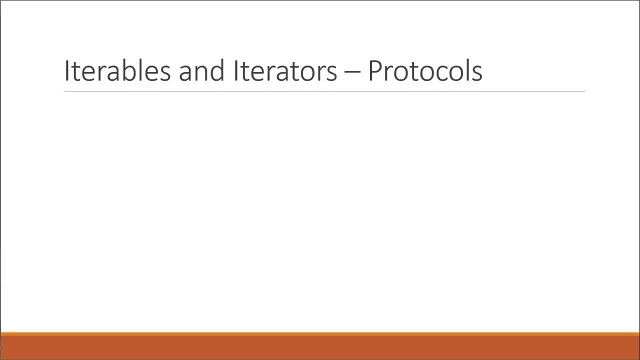 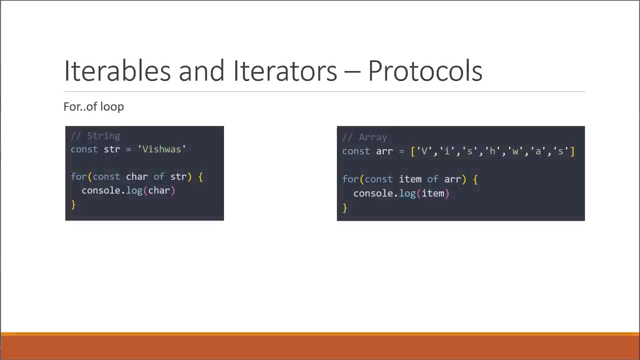 They are termed as built-in iterables, and a new looping construct, which is the for-off loop, was introduced to iterate over an iterable. Here is how the loop works with the same string and array. As you can see, we don't really have to worry about accessing the element from the data. 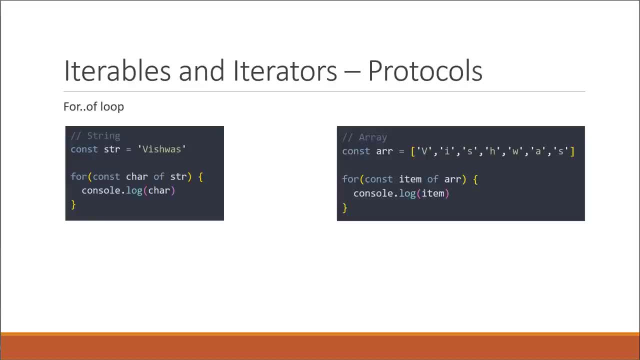 structure. It is just given to us one by one in a sequence, allowing us to focus on the functionality. Of course I'm just logging the value to the console, but you can add any functionality you want to. But clearly this is better than creating a variable. i tracking its. 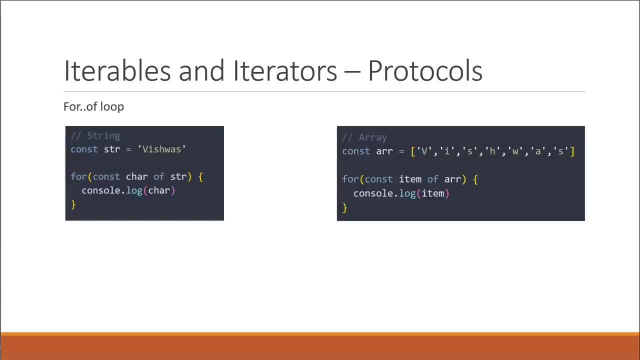 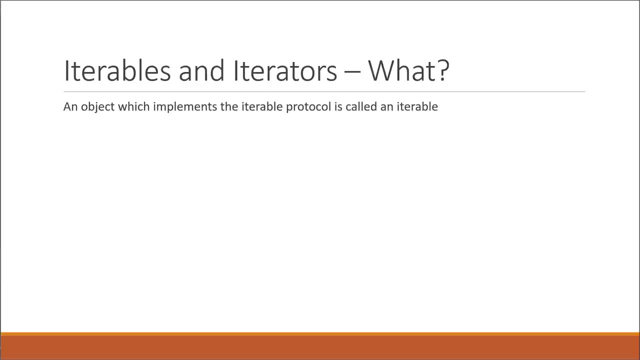 value and checking conditions before accessing the next element. But what exactly is an iterable? Let's understand that now, An object which implements the iterable protocol is called an iterable. Well then, what is the iterable protocol? It states the following: For an object to be an iterable, 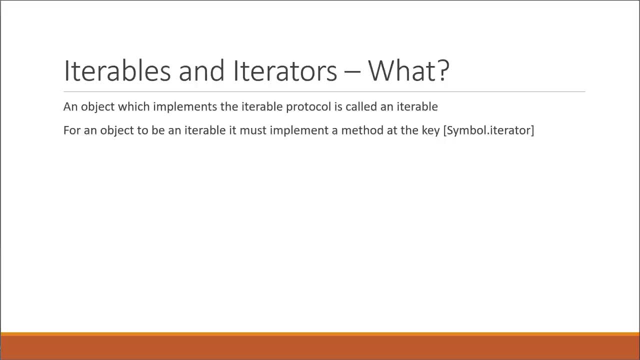 it must implement a method at the key symbol dot iterator. That method should not accept any argument and should return an object which conforms to the iterator protocol. … …, …, …, …, …, …, … … …. Which now leads us to the question: what is the iterator protocol? 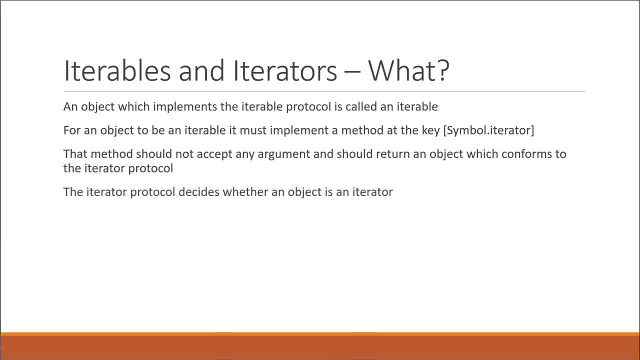 The iterator protocol decides whether an object is an iterator. An object is an iterator when it satisfies the following rule: The object must have a next method that returns an object with two properties: Value, which gives the current element, and done, which is a boolean value indicating whether 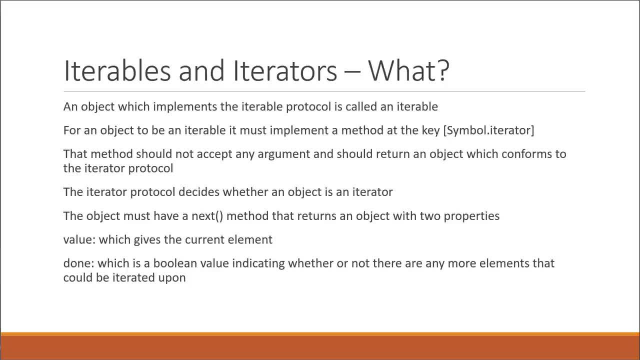 or not there are any more elements that could be iterated upon Now. if this made no sense whatsoever, don't worry, because I was on a similar boat when I started on this topic, And for me what helped was implementing my own simple iterable and iterator. 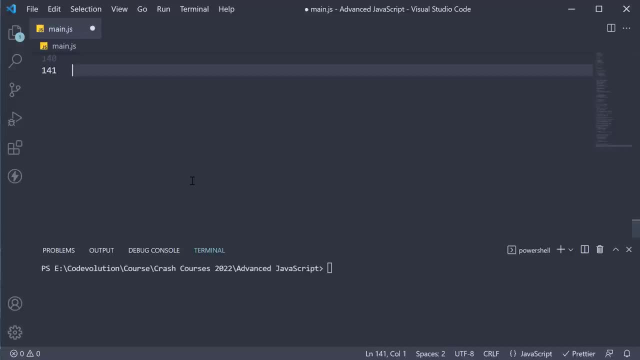 Let's head back to VS Code and do just that. Consider an object which is not a built-in iterable. So const obj is equal to an empty object. Our goal is to make this object an iterable so that when this object is used with the 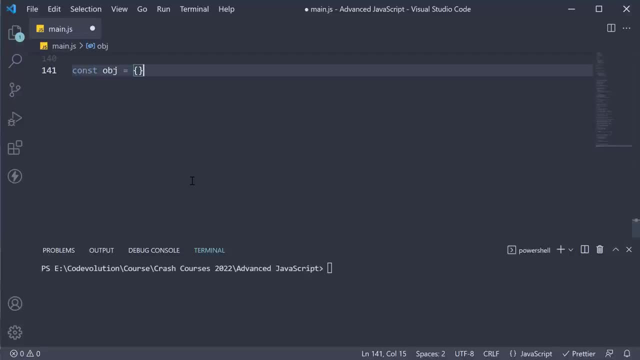 for-of loop. it will print hello world one word at a time. For an object to be an iterable, it must implement a method at the key symbol, dot iterator. So let's head back to VS Code and do just that. Consider an object which is not a built-in iterable. 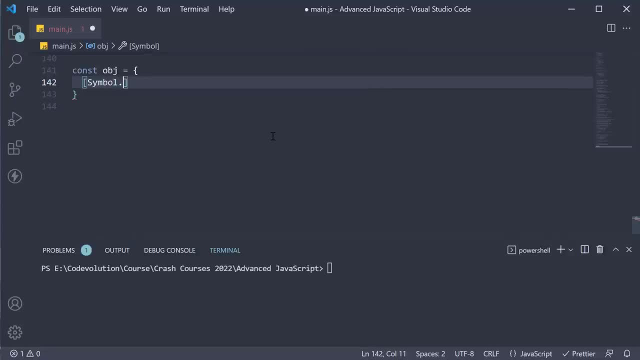 So const obj is equal to an empty object. Our goal is to make this object an iterable, so that when this object is used with the for-of loop, it will print hello world one word at a time. For an object to be an iterable, it must implement a method at the key symbol: dot iterator. 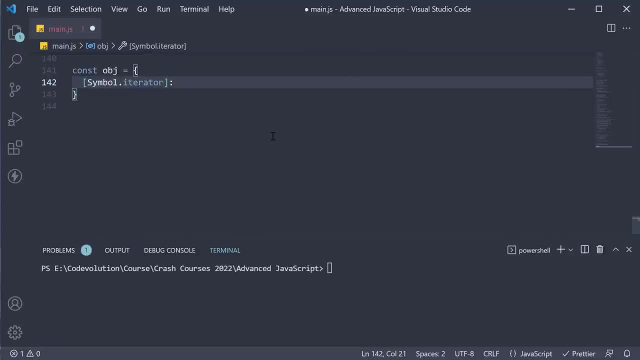 So add a key symbol dot iterator and add this key symbol dot iterator. The final rule of the iterable protocol is that this method should not accept any argument and should return an object which conforms to the iterator protocol. At the moment, we don't know much about what an iterator is. 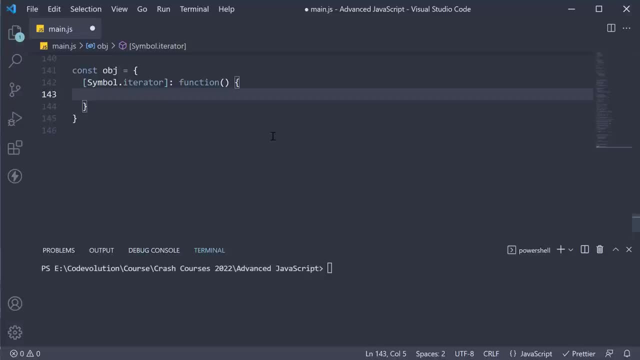 But we do know it's an object that implements the iterator protocol. So I'm going to create an object called iterator and then return it Const. iterator is an object and I'm going to return iterator. This is pretty much the iterable protocol expressed in code. 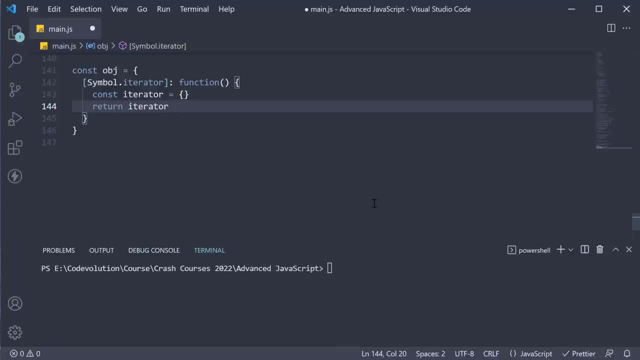 Next, we need to implement this iterator Now. an iterator is an object. It's an object that has a method at the key. next, The method should return an object which contains two properties- value- and done So in the iterator object. we're going to define a method at the key next. 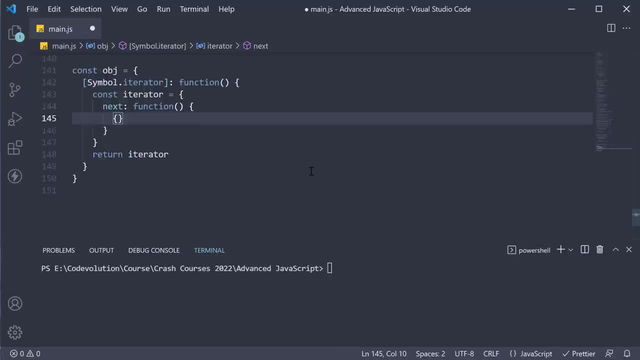 And this method will return an object which contains two properties: value and done. Value gives the current element, and done is a Boolean value which indicates whether there are more elements to be iterated upon. I'm currently not returning the object on line 145, because this is where we need to come up with our logic. 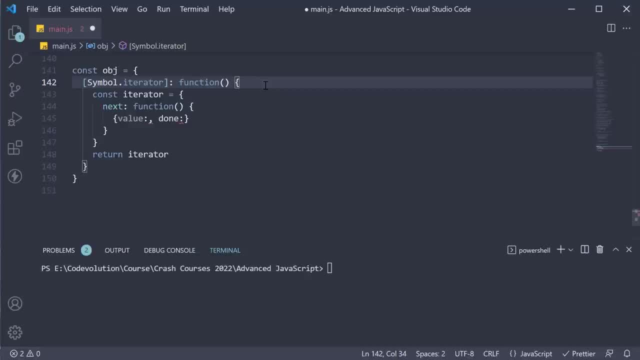 So within the outer function defined at key symbol dot iterator, we declare a variable called step and initialize it to zero. Within the inner function, we increment the value of step by one And, based on the value of this step variable, we return the appropriate object. 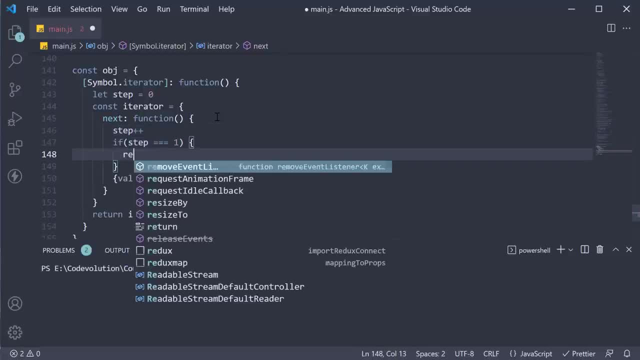 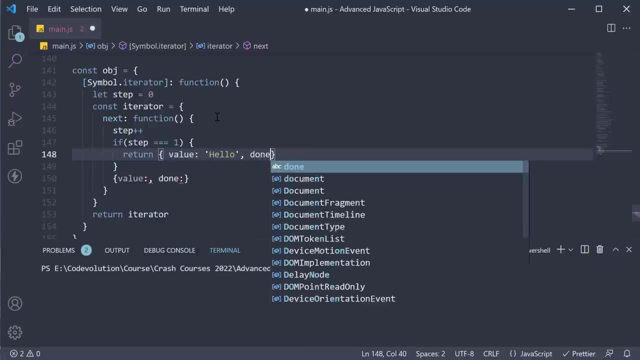 If step is one, we return an object where value is going to be the string hello and done is set to false. Similarly else, if Else, if step is equal to two, We're going to return a similar object where value is world. 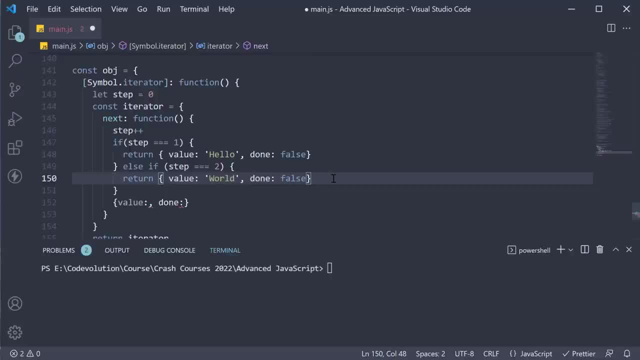 And done is still false. So for step one and two we returned hello and world and done is set to false. When step goes beyond two, we return undefined and done is set to true. So return an object Where Value Is. 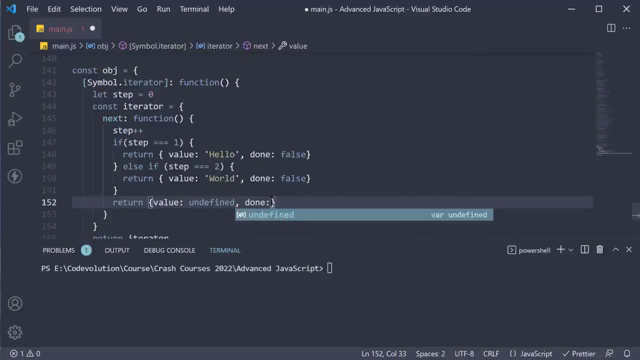 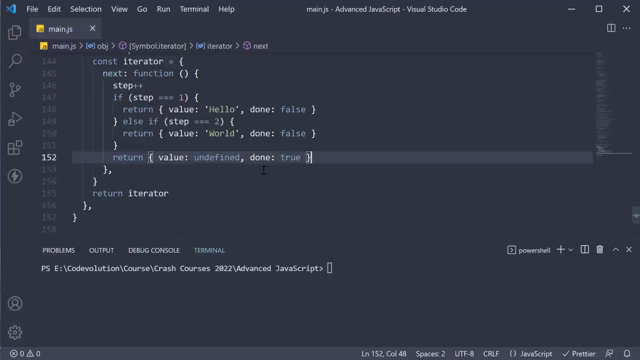 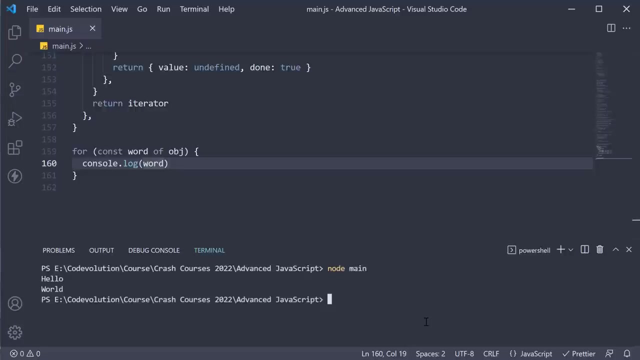 Set to true is undefined and done is set to true. so we are saying there is no more iteration necessary if we now use this object with a for off loop. so far const word of OBJ console log word run, node main. you can see it locks the value hello, followed by world. our object is now an iterable, to be more. 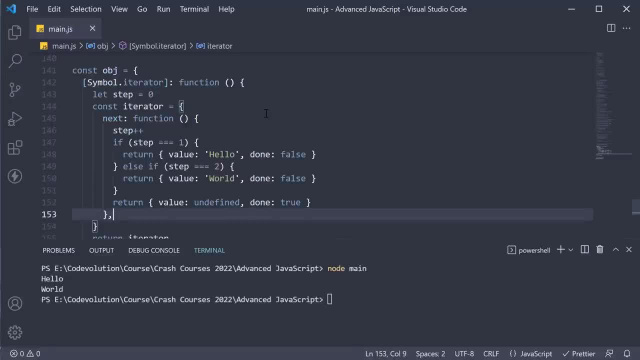 precise, we have created our very own iterable now, similar to what we have done here. JavaScript does it internally for strings, arrays, maps and sets. that is how you can easily iterate them with the for off loop. hopefully, you now know what are iterables and iterators in JavaScript. 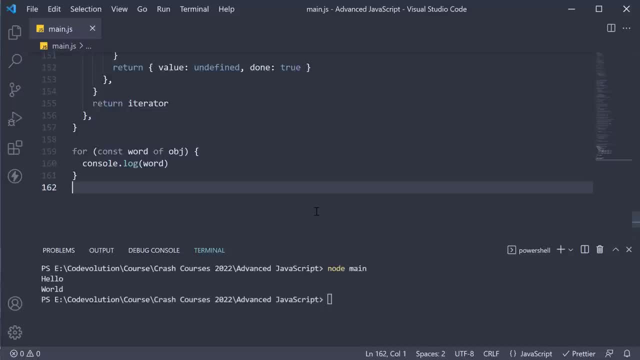 all right for the last topic in this advanced JavaScript crash course. we're going to learn about generators. we've just seen how to create our very own iterable and iterator. even though it is not difficult to make an iterator ourselves, that is, create an object with the next method and define its behavior- it is definitely a verbose implementation, wouldn't? 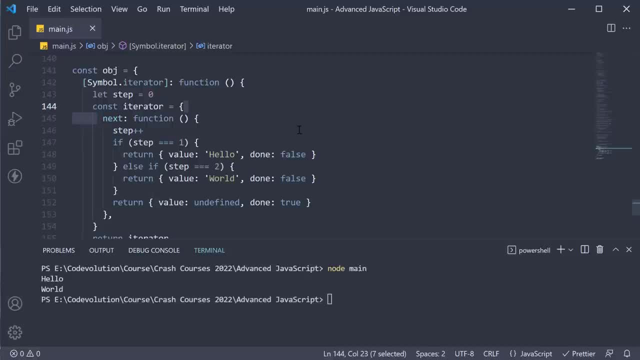 it be nice if there was something that would create an iterator for us instead of us having to write it. that is where generators come into picture. generators are a special class of functions that simplify the task of writing iterators. now, there is a lot to learn about when it comes to generators, but for this crash course, we're only going to focus on the part where 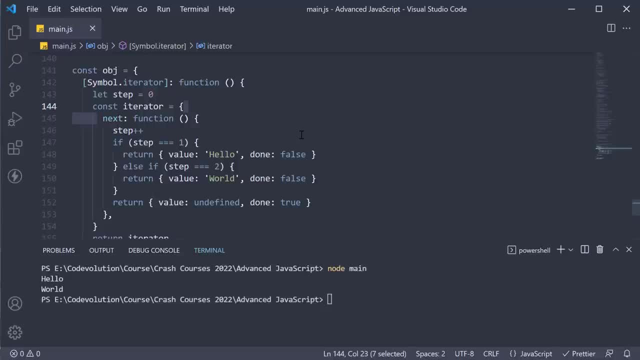 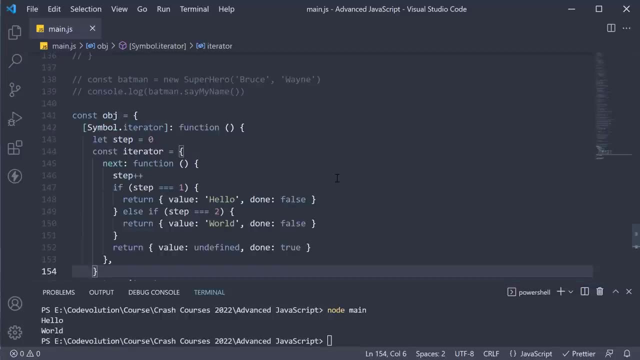 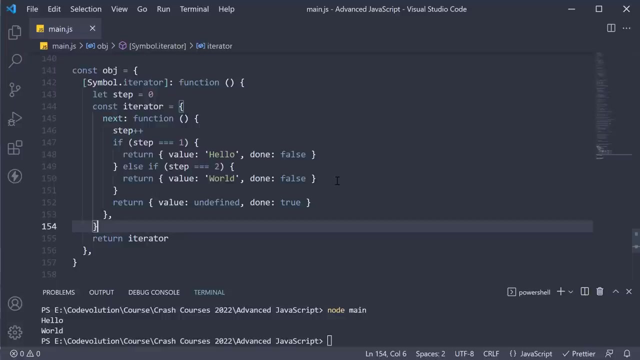 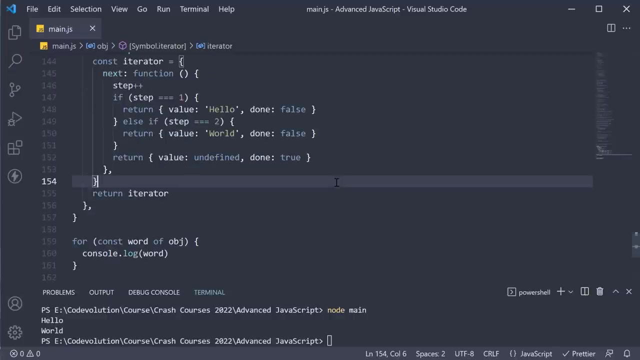 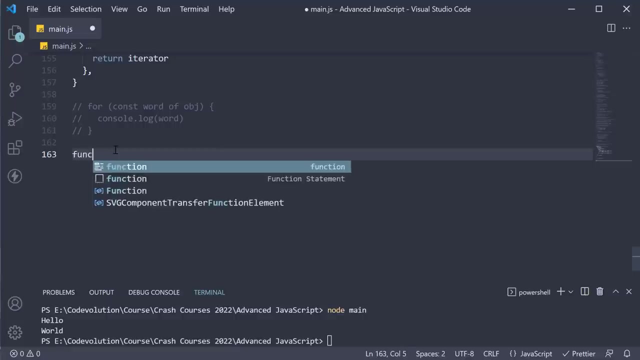 it relates to iterators in JavaScript. in fact, what we are going to do is rewrite this very hello world example using generators. that will allow you to compare and contrast writing our own iterators versus using generators. all right, so how can we create a generator in JavaScript? we write functions using the function keyword, so function. 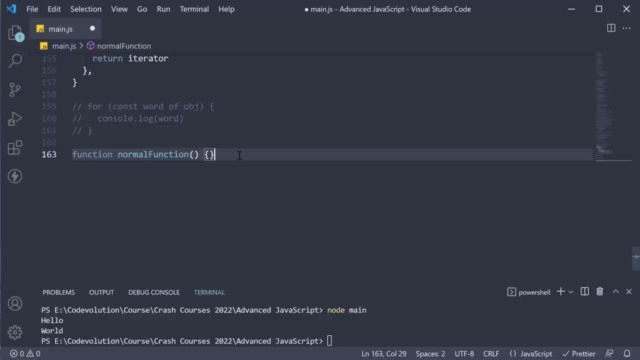 normal function- parentheses and curly braces- a generator. since it is a special function, we use the function keyword, followed by an asterisk function: asterisk generator function- parentheses, curly braces. but what is so special about it? now, we all know that a normal function follows the run to completion. 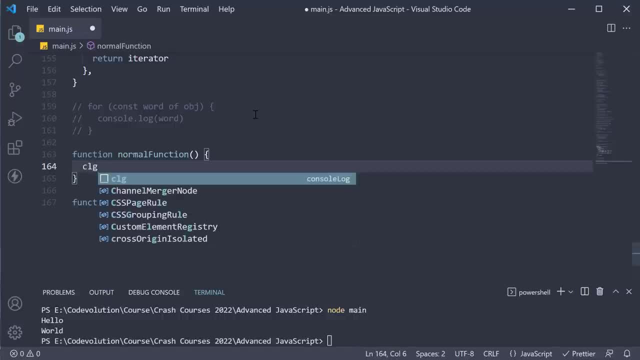 model. so if I add two log statements to log hello and world, this normal function, what we have here, will not stop before the last line is executed. the function will log hello, followed by world, to the console. the only way to exit this function is by returning from it or throwing an error. 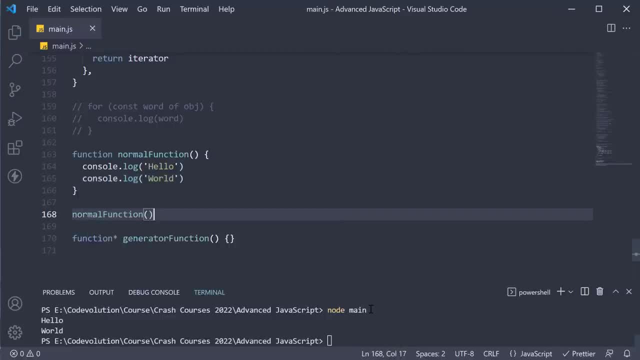 so if we call normal function and run node main, we see hello and world. if you call the function again, it will begin execution from the top. we see hello world and hello world. in contrast, a generator function is the function that can midway and then continue from where it stopped. or you could say a generator. 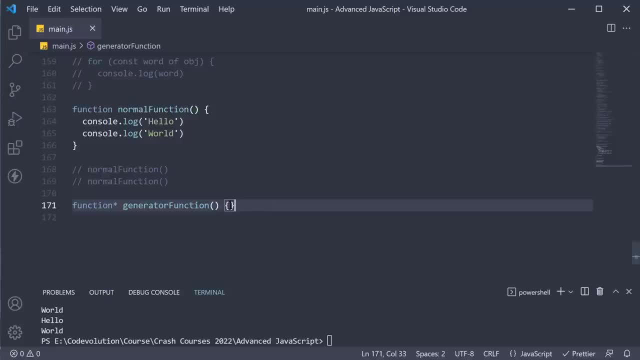 function can pause the execution. to achieve that behavior we use the yield keyword, so yield hello, and in the next line yield world. yield is an operator with which a generator can pause itself. every time a generator encounters a yield, it yields the value specified after it. we don't say it returns a value. 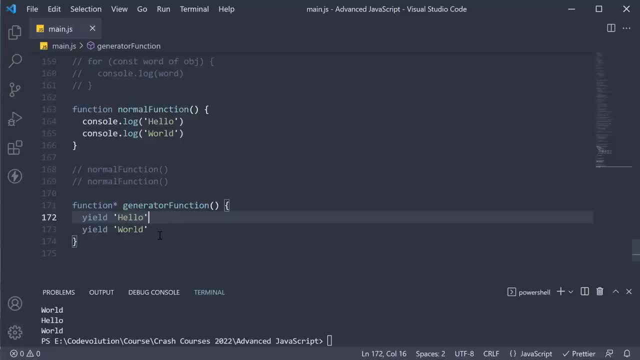 we say it yields a value. next let's talk about invocation. we invoke a generator function by adding parentheses after the function name, so generator function and parentheses. however, unlike returning a value from a normal function, a generator function always returns what is called a generator object, so const generator. 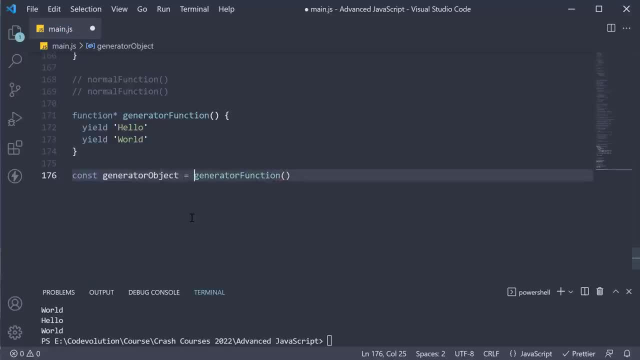 object is equal to the invocation of generator function and this generator object is an iterator. so instead of us having to create an iterator, a generator function will create it for us and because the generator object is an iterator, it can be used in for of loops. so for const word of generator object, log to the console word. if we clear the. 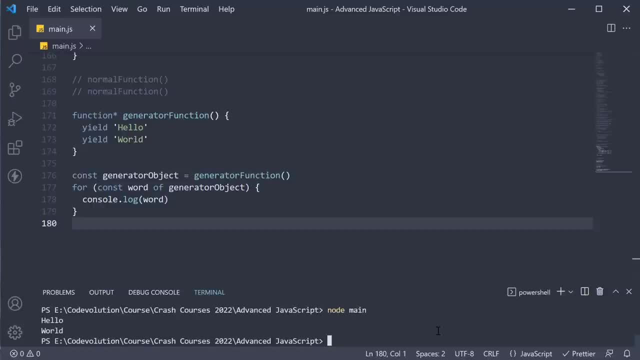 terminal and run node main, you can see hello, followed by world. as you can see with generators, we not only have created an iterable that returns hello, followed by world, but we also have a simpler way to create iterators. we have achieved the same iteration behavior. we had seen two.